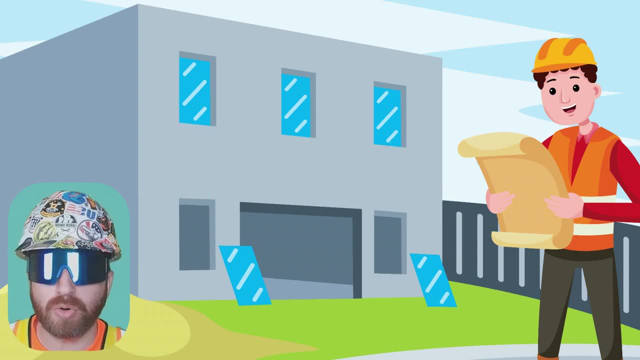 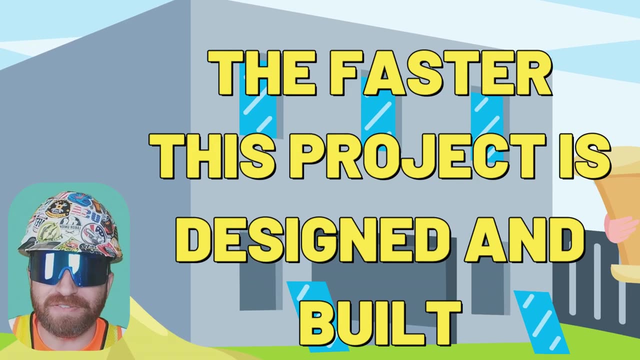 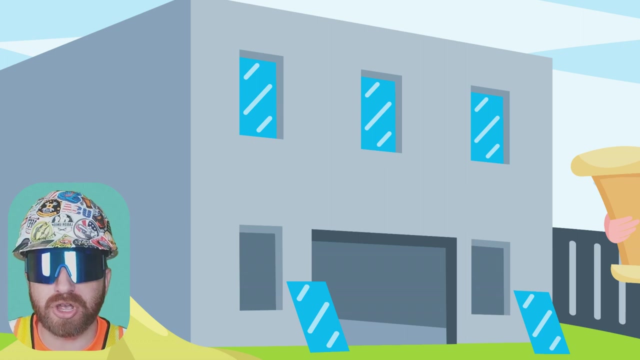 and potential profitability from that project. The owner is also going to be looking for a schedule as part of their consideration to take this idea to actual construction. So the faster this project is designed and built, the faster the owner receives their return on their initial investment. So schedules are just as important to owners as project costs are. 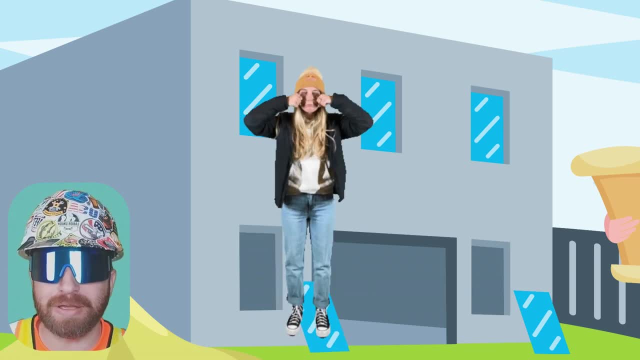 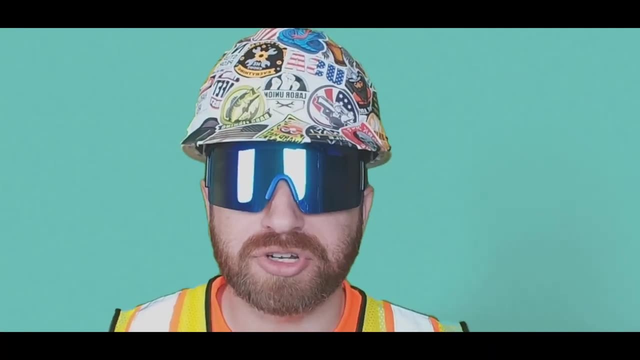 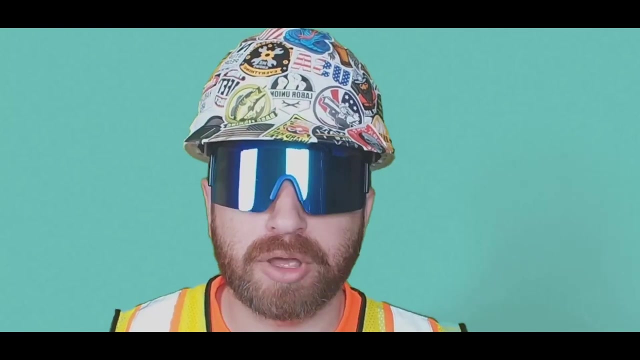 because the cost of a building sitting incomplete could financially impact this owner, who is not earning profits on the building when they potentially could or should be. So this is why commercial construction contracts are typically, and most often, written with defined project completion dates, Whether there are liquidated damages or other consequential 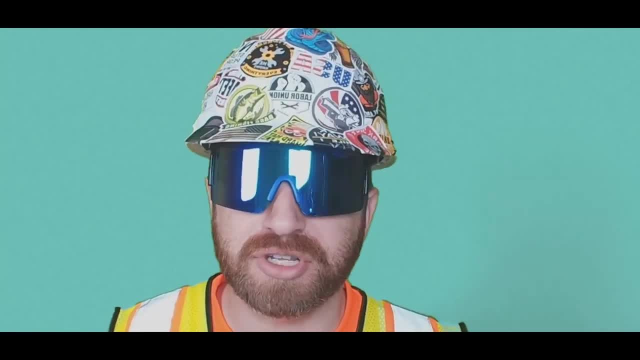 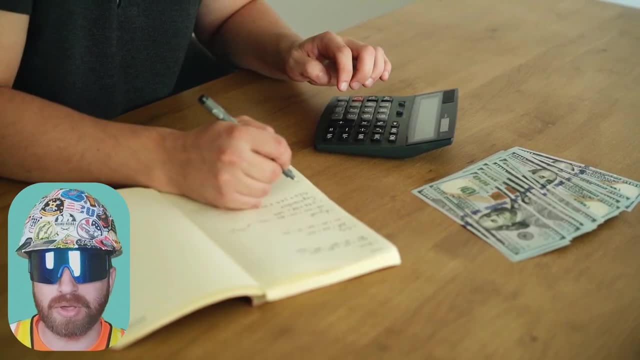 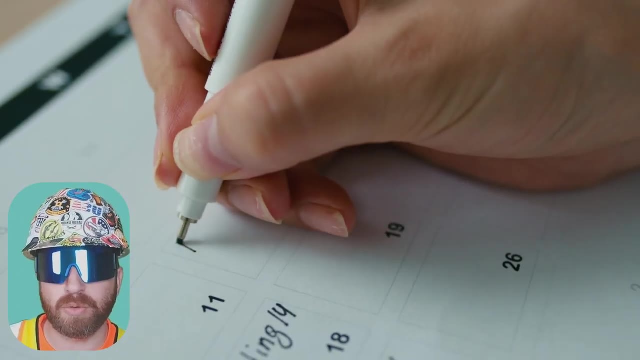 damages incorporated and tied to those completion dates is just another topic for another day. So just as a general contractor can provide a square foot price estimate of a building in or conceptual phases of construction based on previously completed projects of a similar scope, they can do the same thing with a schedule, For instance. let's say we know the owner. 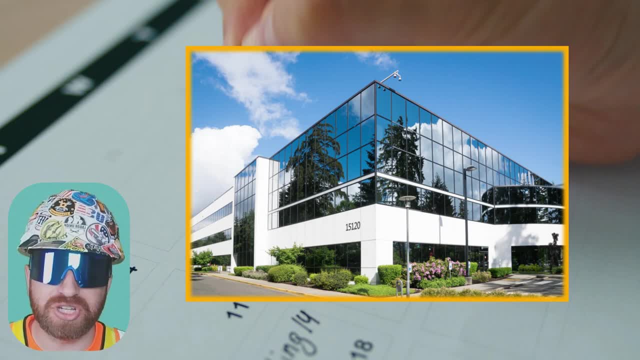 wants to build out a commercial retail space and we, as the GC or CM, are given the approximate square footage of this potential project. Well, we've recently completed three similar projects at a similar square footage. We can compare the timelines of those previous projects. 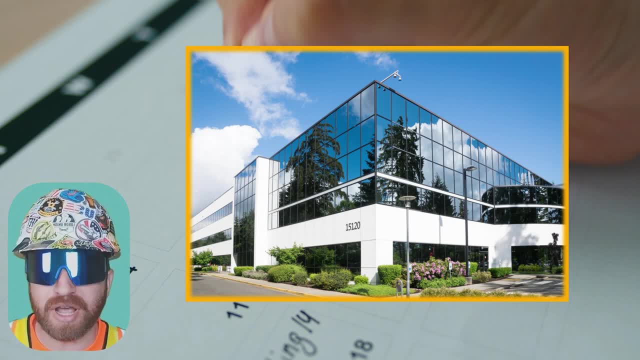 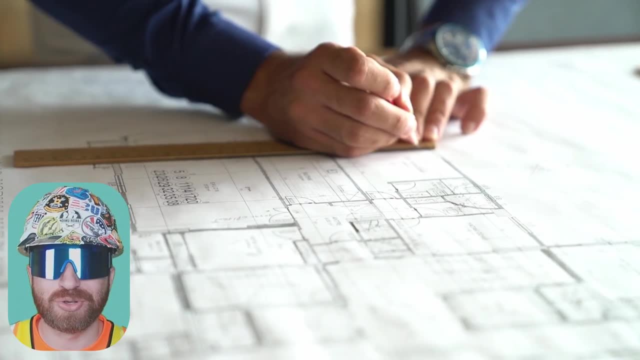 as well as incorporating new variables that we may know, and this is just another example of how a project can be built. This is how we would generate a rough schedule or overall duration of this project to help inform the owner's decision making. So as design continues, we start to understand more, and 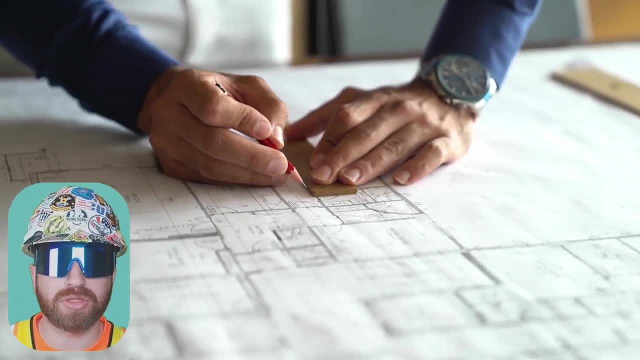 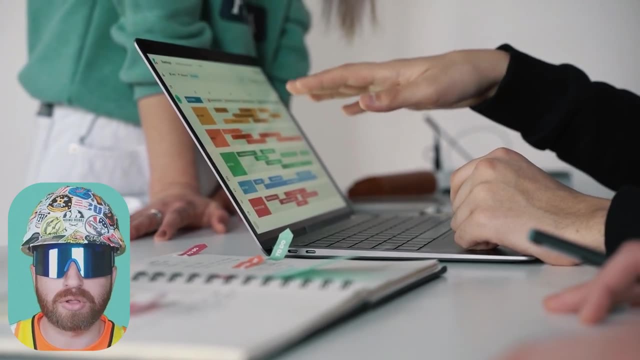 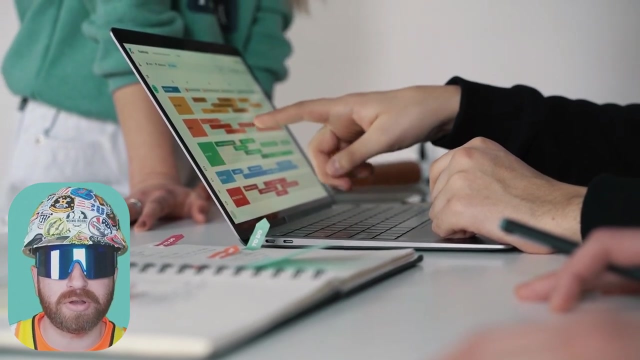 more specifics to the project. Thus, we can refine the budget through conversations with key subcontractors, as well as refining the schedule through these same conversations. The closer a GC or CM gets to compiling final bid documents, the more refined the schedule should become, with clear expectations and milestone dates. 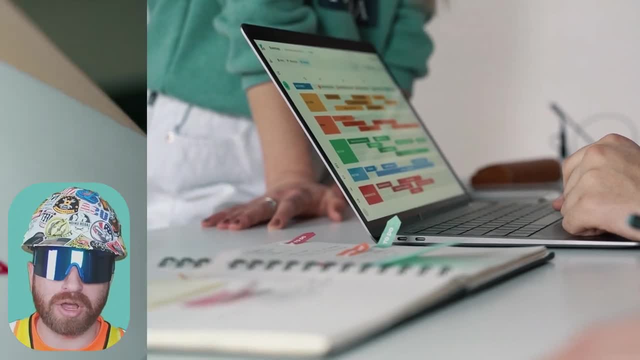 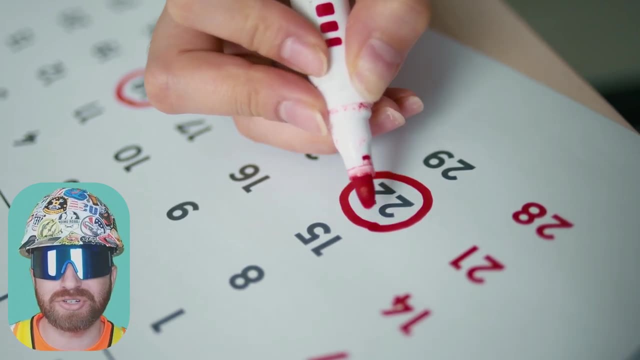 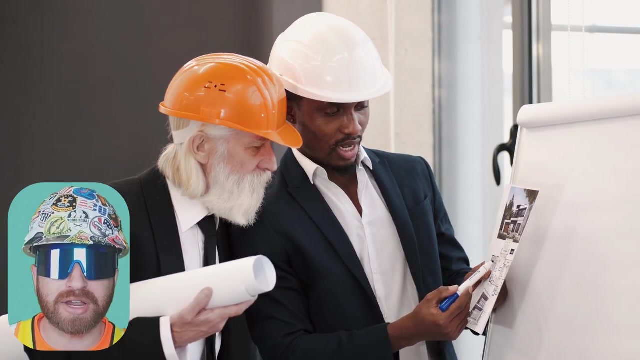 And then, at this point, the schedule starts to shift from what was broad durations to now incorporating these milestone dates as well as specific activities. General contractors and construction managers work out a presentable and manageable schedule, which ultimately gets incorporated into the bidding documents that all contractors will. 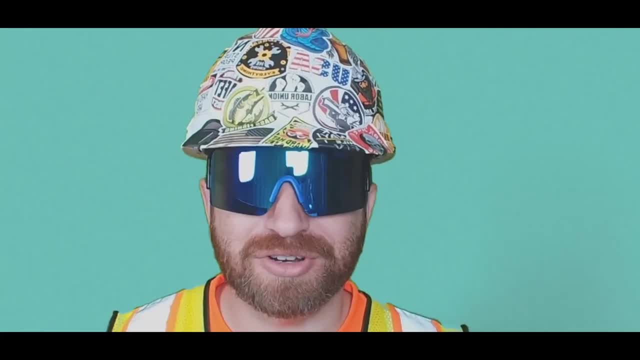 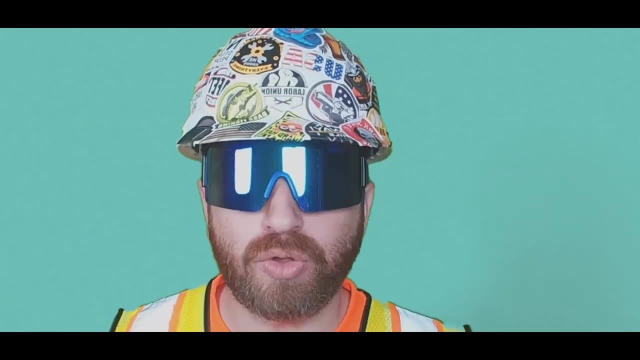 be submitting their pricing against. So when general contractors, construction managers, trade contractors and subcontractors are bidding on commercial construction projects, they're not only committing to certain budgets, but they're also committing to certain schedules, site logistics plans and other contract documents that they've all reviewed and 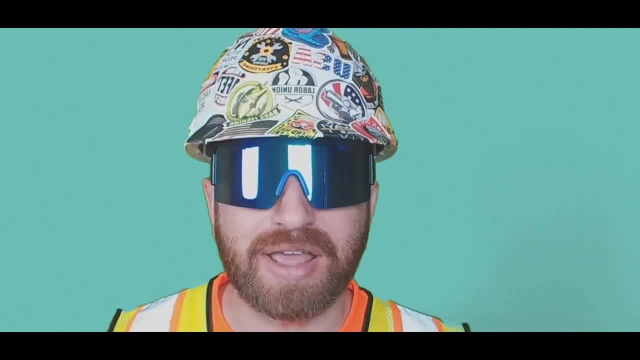 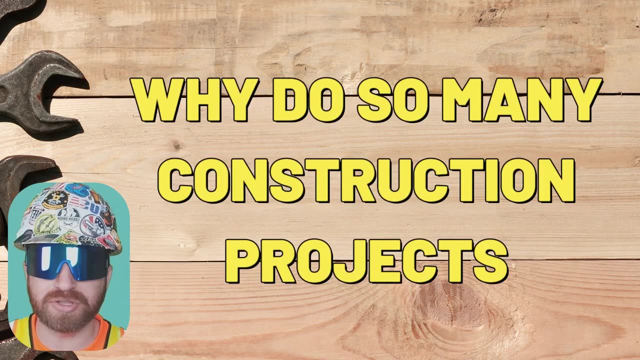 said: yes, we all agree we can do this and meet these parameters. So let's pause here for a moment and talk about why so many construction projects seem to have highly aggressive schedules, meaning shorter timeframes. Now, at some point, every individual 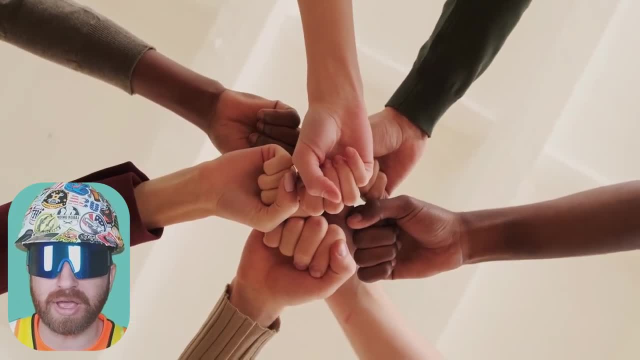 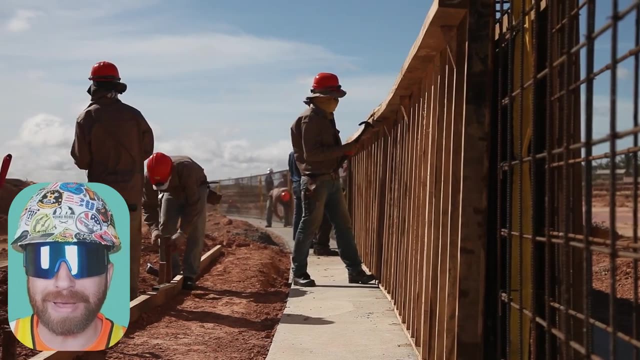 or company working on any given project agreed and bought into some baseline schedule prior to committing to that project. However, through time, each project will have an individual or company working on a specific schedule, which means that each project will have an individual or company. 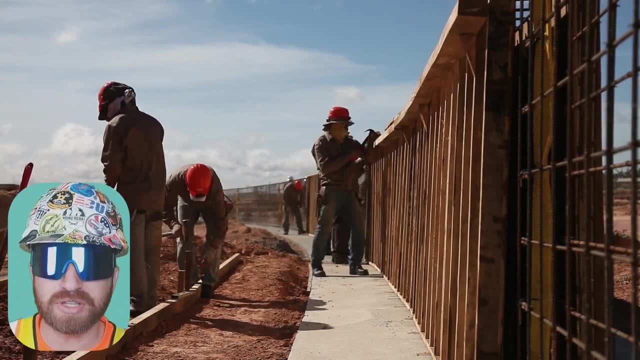 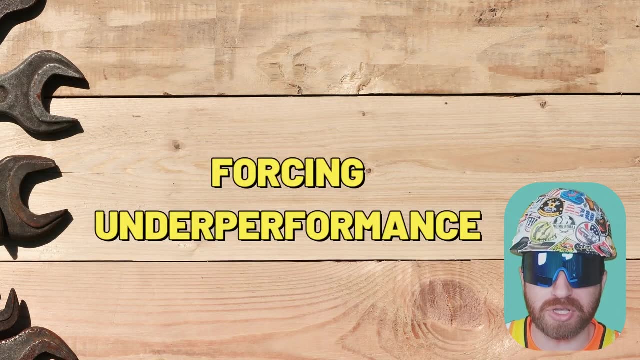 working on a specific schedule prior to committing to that project. However, through the competitive bidding process, it continues to not only pinch profits, but also these scheduled durations, forcing these schedules to be shorter and shorter. So the bigger question is: how many companies are? 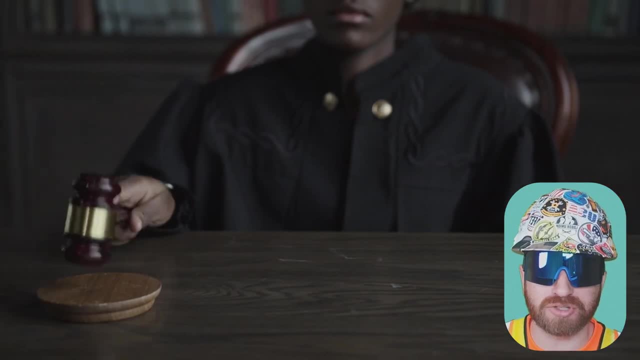 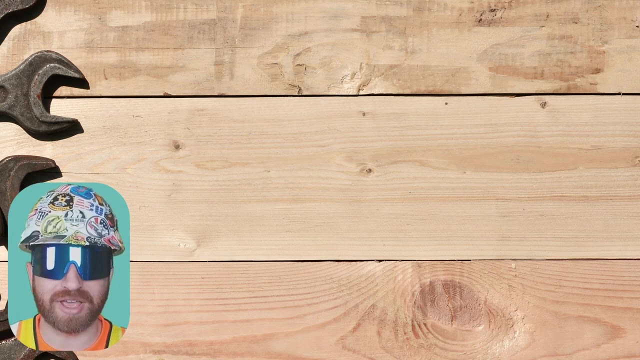 overcommitting and therefore forcing underperformance and failure through this bidding process. We hear so many projects in the news getting into lawsuits because they've missed their turnover dates. Again, a good discussion for another day. The general contractor, construction manager, establishes a bid documentation for the. 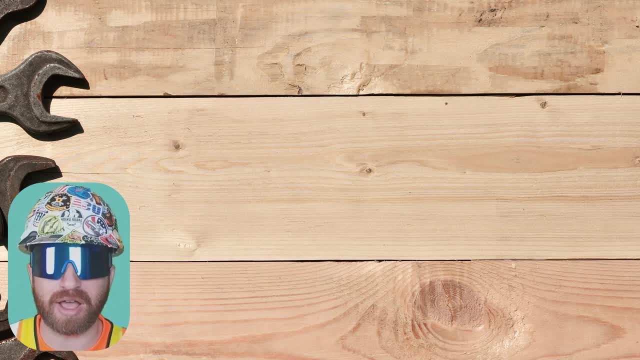 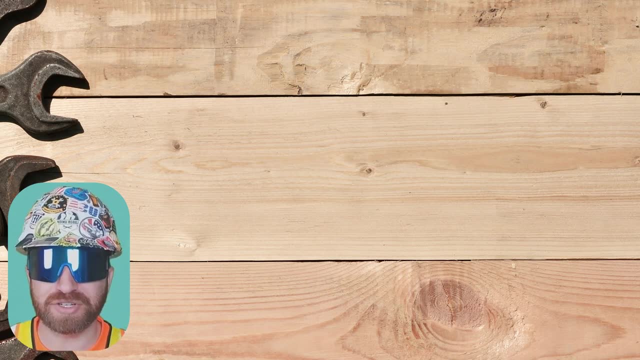 project, which is done by the general contractor, construction manager, in a set of bid documents to meet the needs of the client while still holding reasonable timeframes that everyone can uphold. So how do GCs and CM's take all this information from past projects? 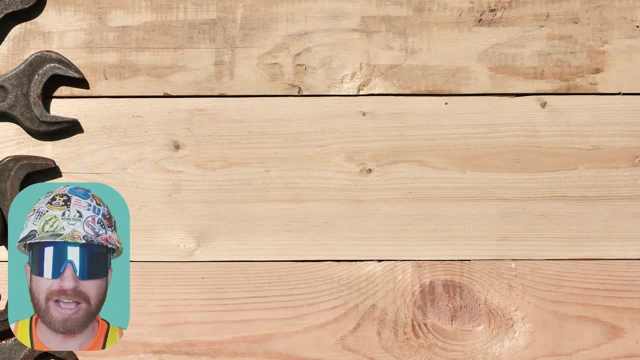 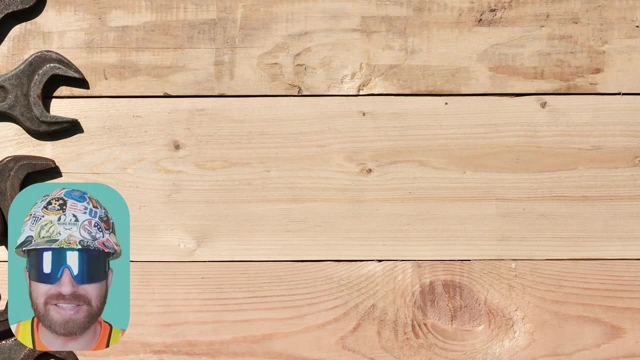 from subcontractors, from this current project scope, combine all this knowledge and generate the most reasonable yet competitive schedule. Well, they all utilize a scheduling practice known as the critical path method, which is the option of using one of the following methods in a project project: 5. Use the загwork shake and start the cycle. then start the cycle. 6. Use the24 hour schedule. 7. Use the 12 hour schedule. 8. Use the 24 hour schedule. 9. Use the membership approach so that the project will be split up. 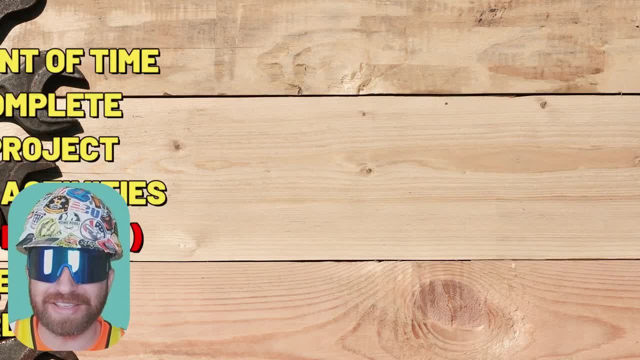 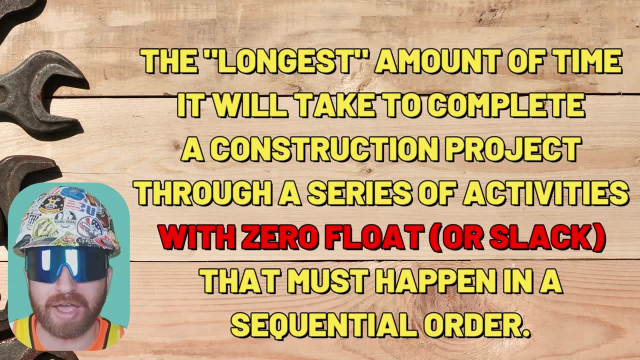 I'm sure you've heard the term used before. The critical path is the longest amount of time it'll take to complete a construction project through a series of activities with zero float or slack. that must happen in a sequential order. Float and slack are interchangeable terms and I'll explain. 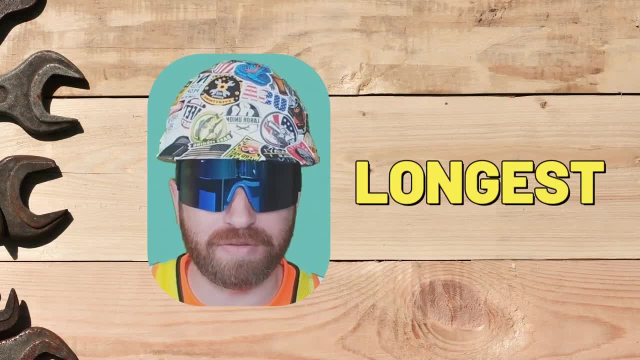 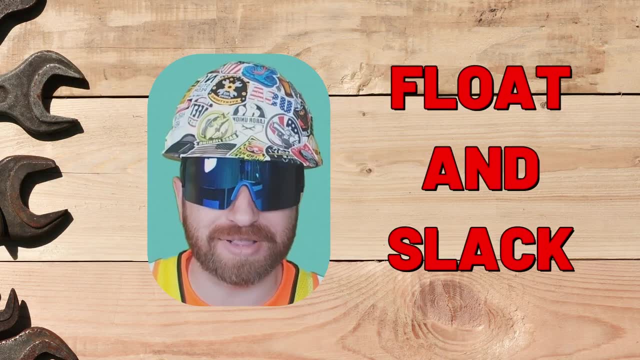 them in just a minute. The term longest in that previous statement confused me when I was first learning about CPM schedules, but the keywords to pay attention to are really float and slack. Also, I don't really think there's a good way to verbally explain CPM schedules, at least for me. 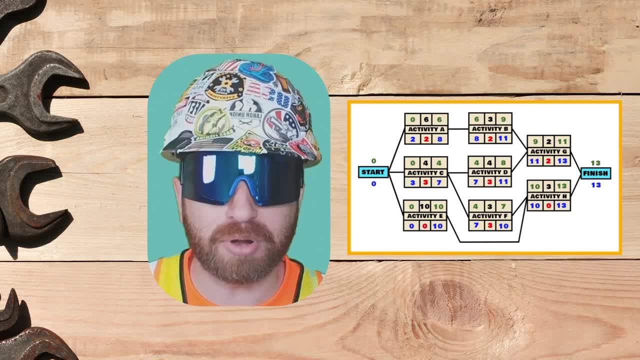 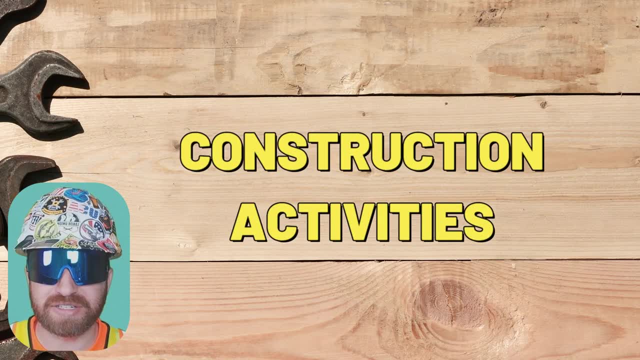 without a good visual representation to go along with it. but I'm going to provide a little more context before we get into that example. So this critical path is based on a series of construction activities that must happen in a sequential order to complete the project. 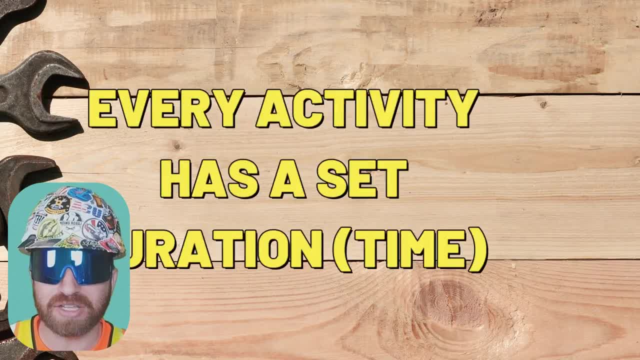 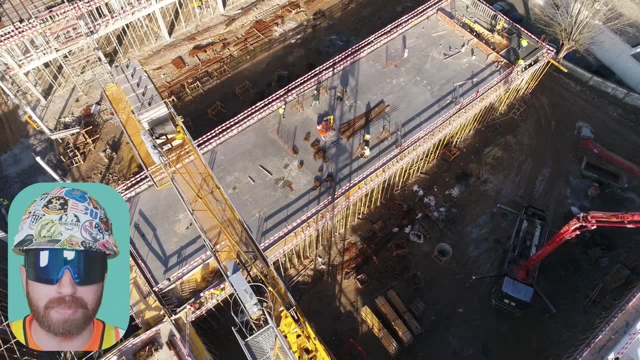 An activity in a schedule is an aspect of scope that has been given a set duration of time, but a construction schedule isn't one path of activities from start to finish. It's multiple paths of activities that originate from one single starting point and end at the. 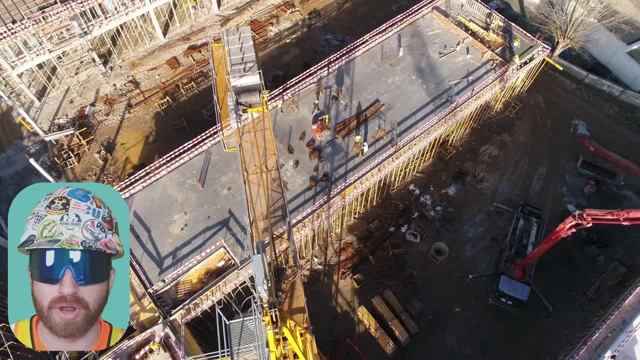 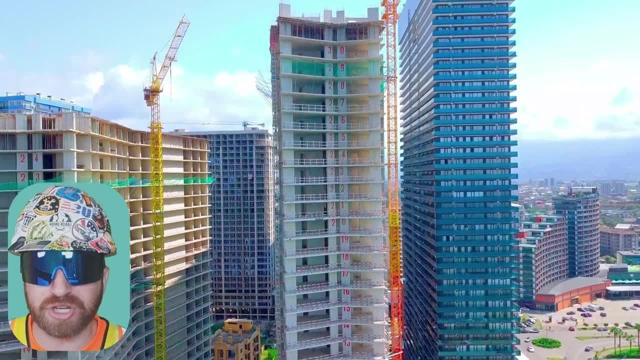 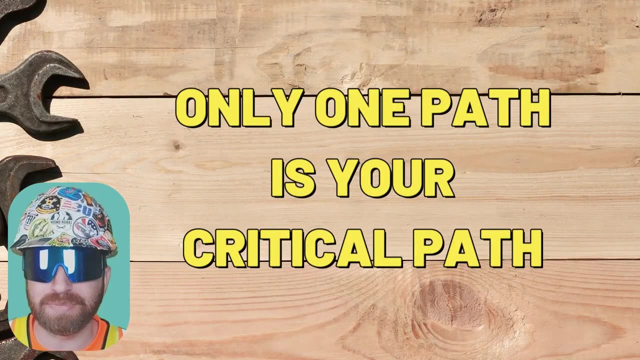 same finish point through a series of relationships with one another. As you know, multiple activities can be happening on a project simultaneously. Activities or scope all have different relationships with one another, based on the sequence of how this building is going to be built. Only one of those paths, though, is deemed the critical path, while the other paths have 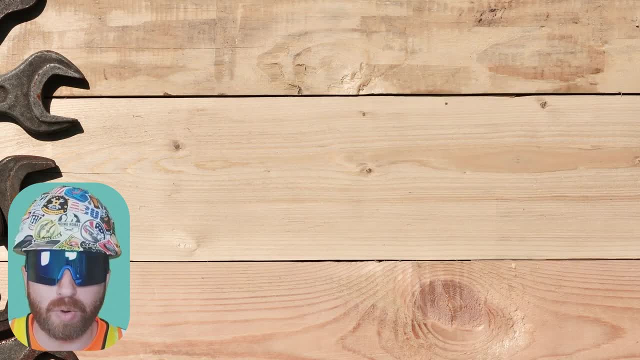 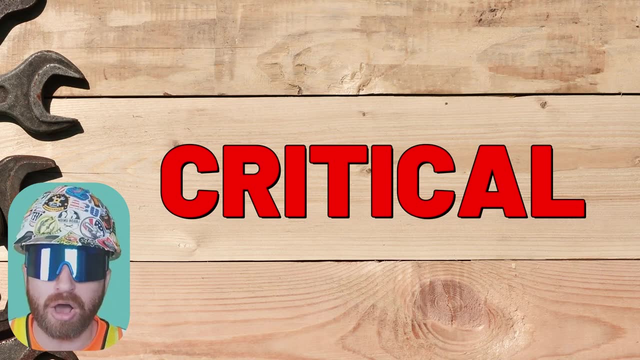 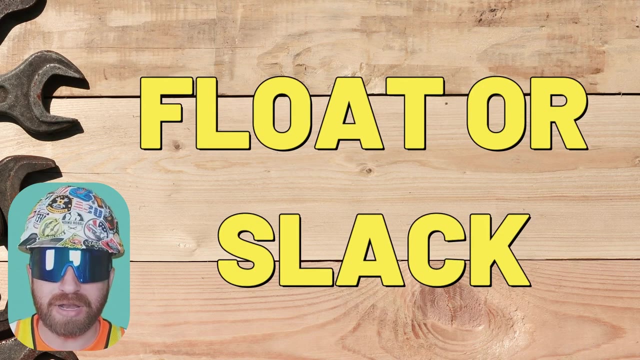 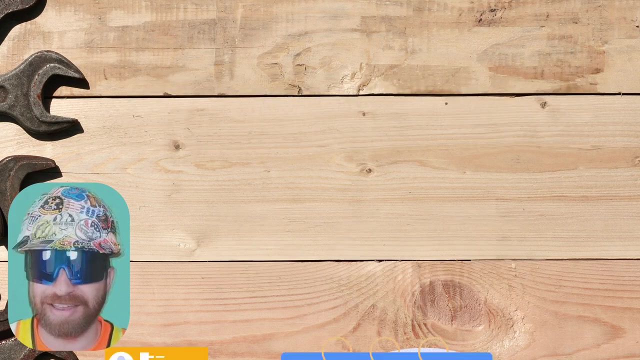 activities that have float or slack. So, to reiterate, activities that are not on the critical path have float or slack, meaning that there could be potentially some hiccups or delays to those activities and the end date of the project will likely be okay. Now, a project schedule is a living, breathing document that 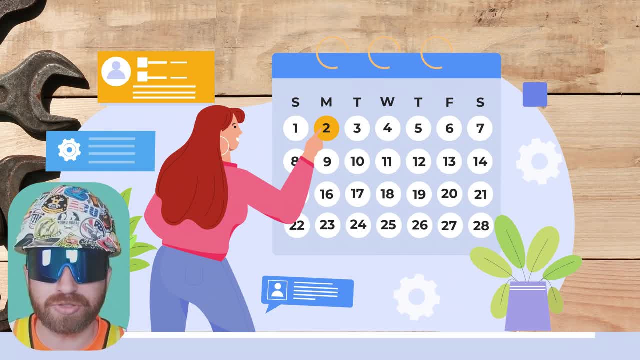 needs regular attention and regular updating to ensure that the project is still on track. The critical path is a project that is not on the critical path but it has float or slack. The critical path can, however, change throughout the duration of a project. 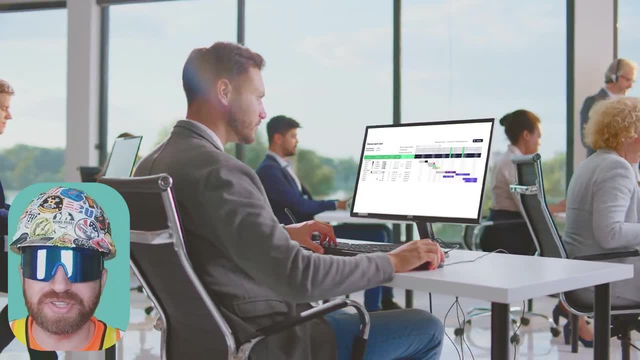 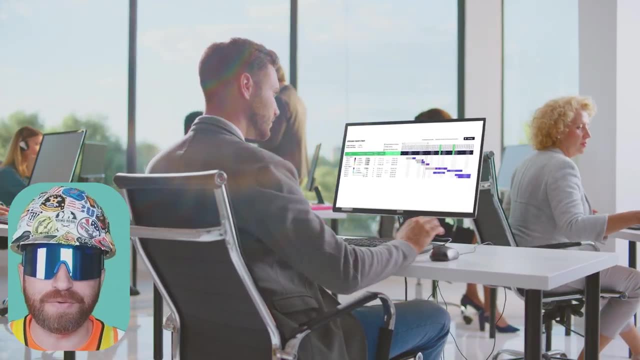 based on these real-time schedule updates. So this schedule is comprised of a start date, a series of activities, potentially some milestone dates, and a finish date. If you recall, an individual activity is any defined scope of work with a set duration. 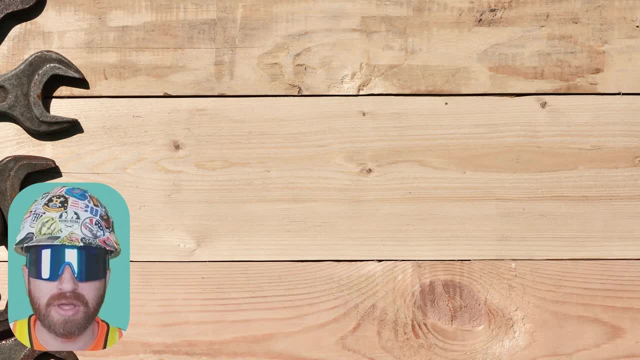 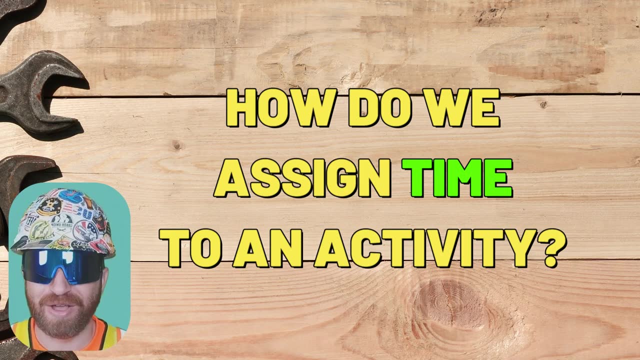 meaning that you have a task and an associated time with it. So how do these activities get their durations defined? How do we know what time to assign to any given project? Well, construction workers, or any worker for that matter, have productivity rates. 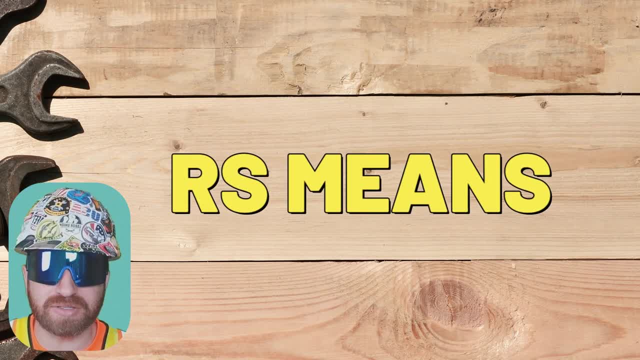 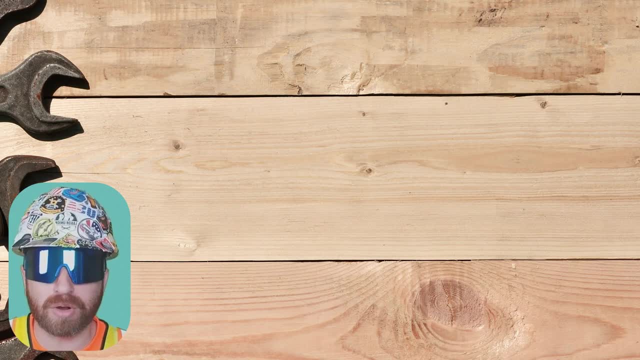 and there are resources online, such as RS Means, that track these productivity rates on a national scale with modifiers based on the city or state that you might be working in. Most companies track their own production rates to ensure that they're building out accurate schedules and budgets on. 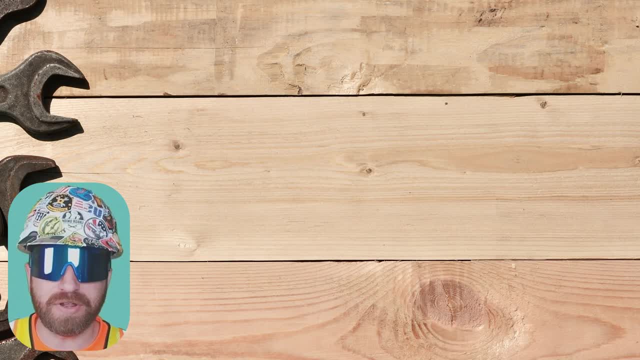 future projects. So let's look at an example of a productivity rate for installing a doorframe and how it relates back to the project. So let's look at an example of a productivity rate for installing a doorframe and how it relates back to the project. 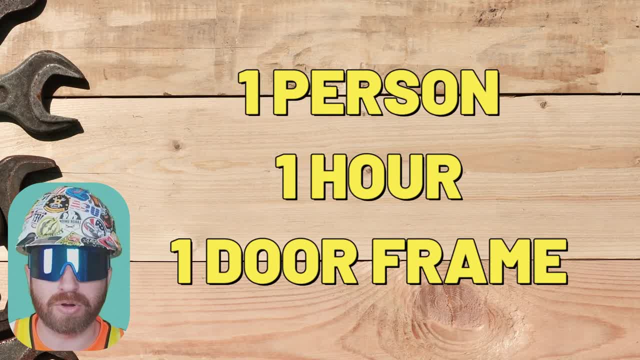 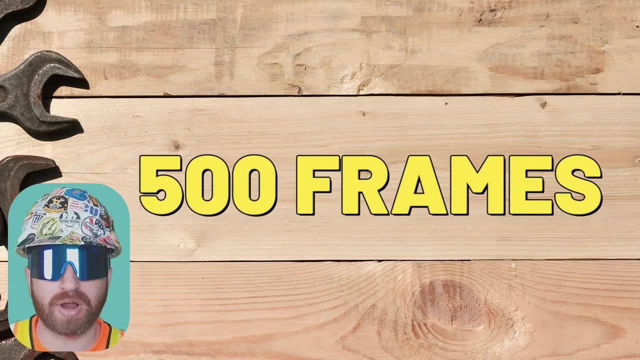 So let's look at an example of a productivity rate for installing a doorframe and how it relates back to the project. Let's say it takes one person one hour to install a doorframe. Well, that's our production rate. Now let's say our estimate captured 500 doorframes on this project. 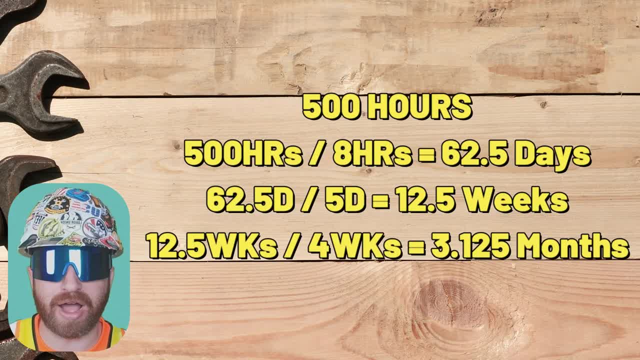 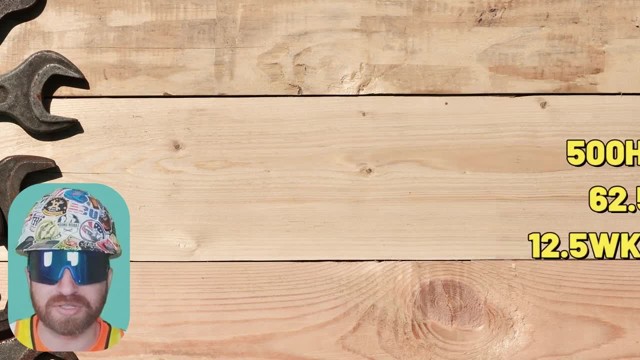 so if we do the math, it would take one person 500 hours to install 500 doorframes, which is the equivalent of about 12.5 weeks or a little bit over 3 months. Well, let's just say that doesn't work out with our overall project schedule needs. 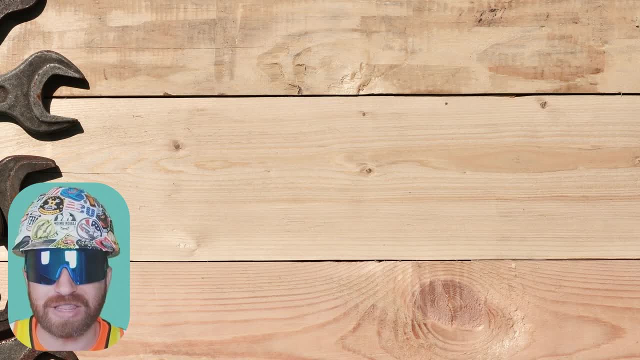 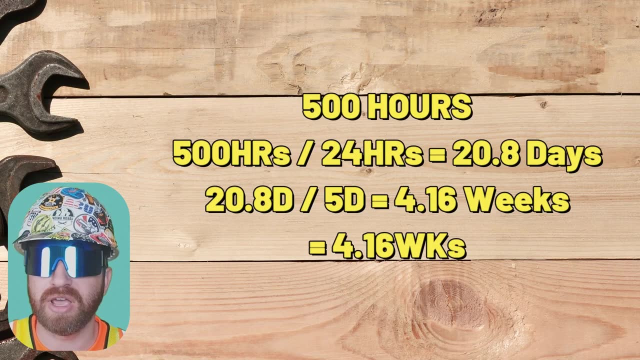 and let's say that we need it done in approximately 4 weeks to maintain the flow of this project. Well, we can't really just adjust productivity in this equation, so the only other thing is crew size If we utilize a three-person crew in lieu of one person. 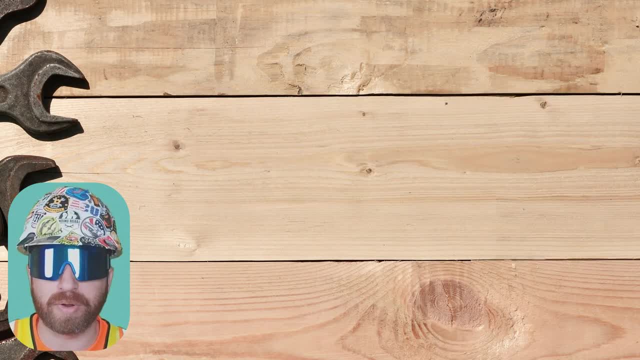 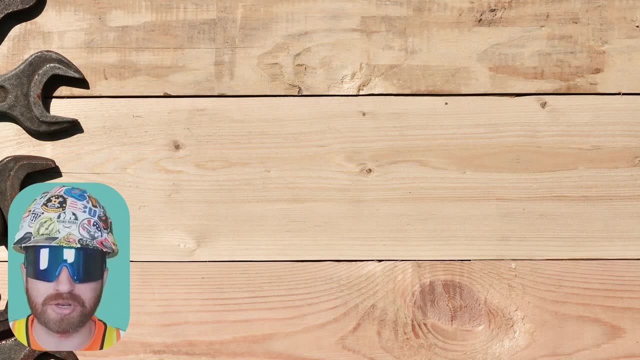 we cut the time by three, Twelve weeks turns into four weeks. Now you won't be doing this on every activity in your schedule, but this is how you would use production rates to generate schedule durations. You'd use this if you wanted to calculate or back check whether durations in your schedule 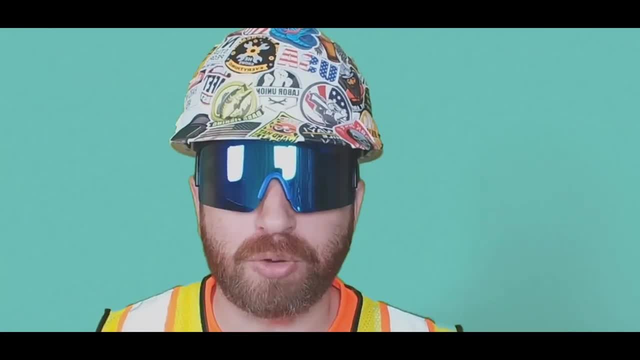 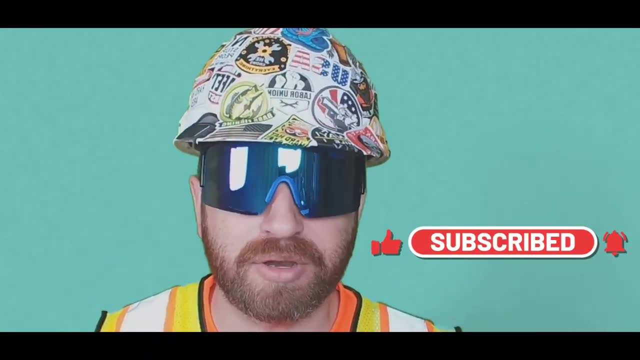 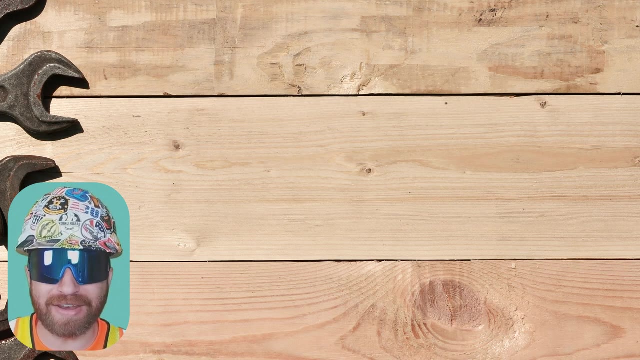 are accurate or not. I'm just sprinkling this into this video because production tracking is directly tied to both scheduling and a future video I'll make in regards to forecasting and profitability of a job, which is the large aspect of project management. So I'd argue that compiling an accurate construction schedule and understanding 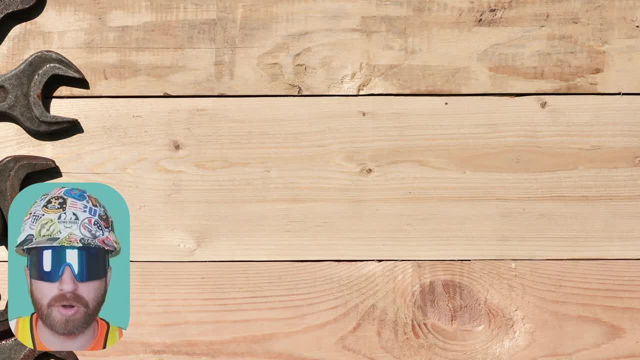 project sequencing is one of the most difficult tasks for a majority of people to grasp when first entering the construction industry. So, just like anything, this is a learned skill that you'll need to work on and develop over time. Project scheduling is your roadmap that influences. 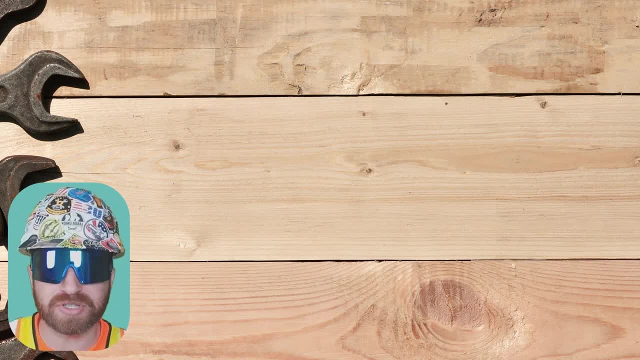 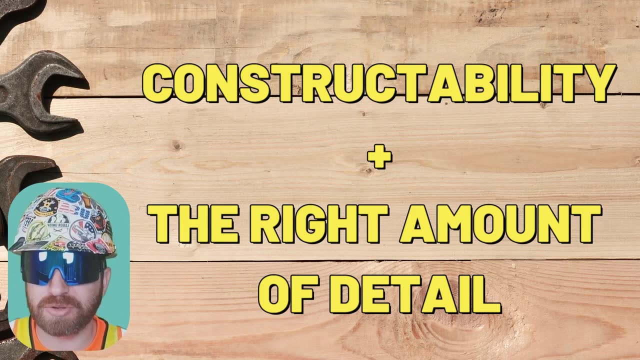 your project. It's not only what your project should be doing today, but what you should be focused on and planning months in advance. Ultimately, the schedule needs to be a balance of having enough information to make sense to be constructible without too much detail that bogs. 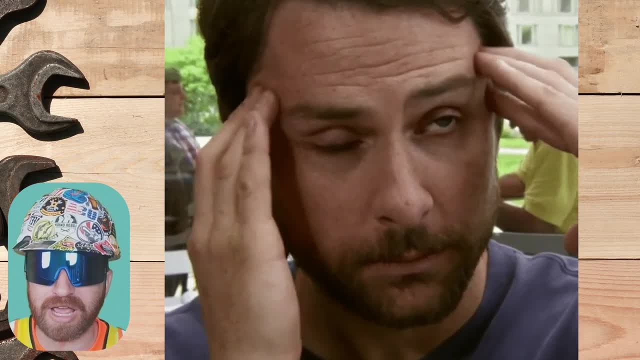 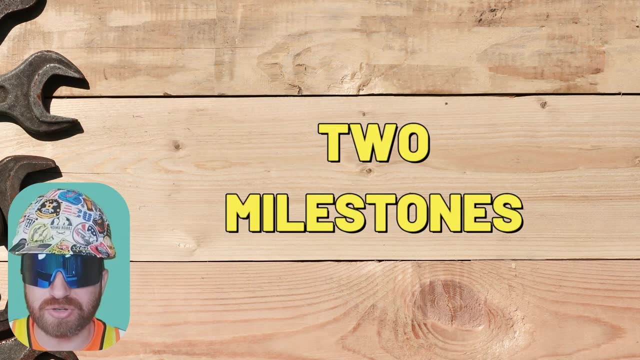 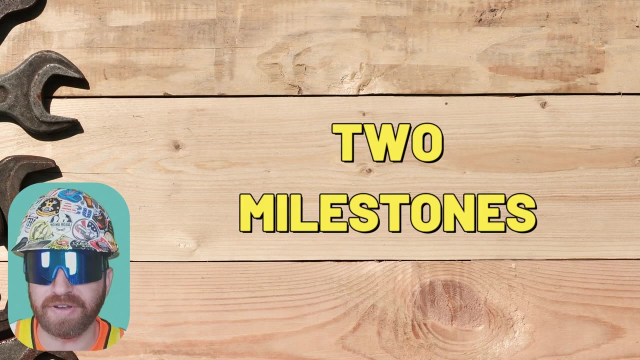 down and confuses people. Too much detail might leave less flexibility to adapt to unforeseen changes when you need to update your schedule or activity relationships in the future. Now every project schedule should have at least two milestones. Milestones are points in zero duration associated with the activity and are there to establish a goal or a target. 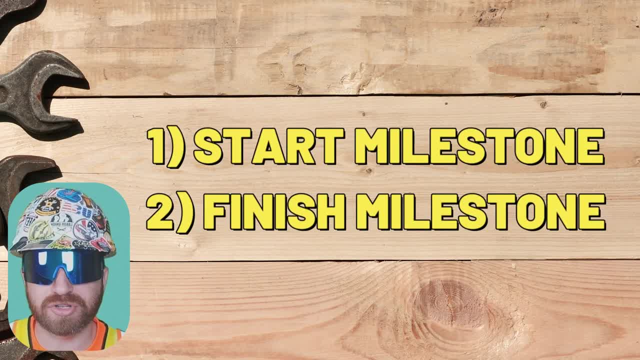 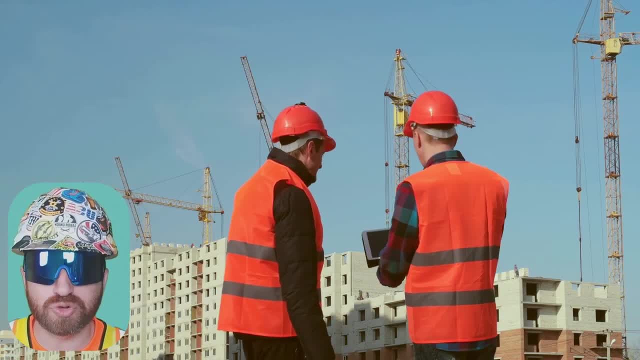 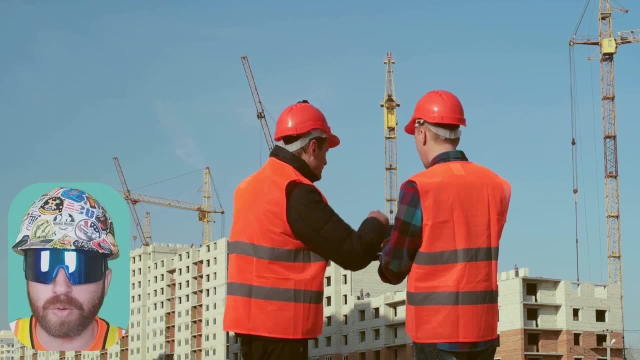 The two milestones every project is going to have will be your start milestone and your finish milestone. Other milestones may include structure being complete, envelope, dry-in, in-wall inspections, above-ceiling inspections, final inspections and more. They're included as a straightforward measurement to determine whether or not the project is on track or not. 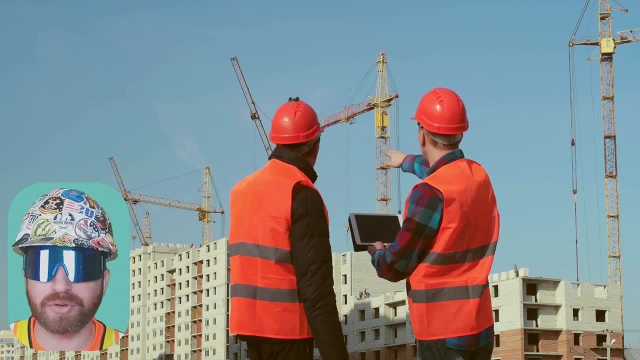 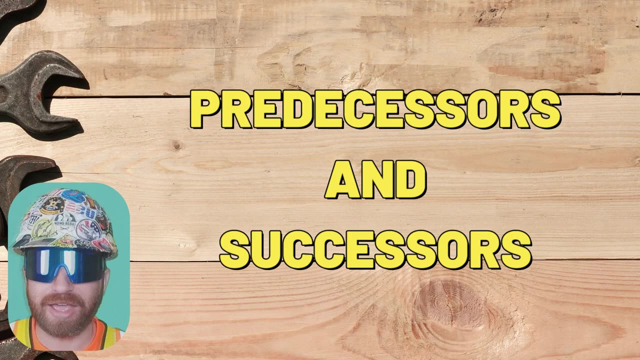 Aside from your start date and finish date milestones, every other remaining activity will have relationships to other activities in the form of both predecessors and successors. A predecessor is an activity that happens before a specific activity. A successor is an activity that happens after a specific activity. 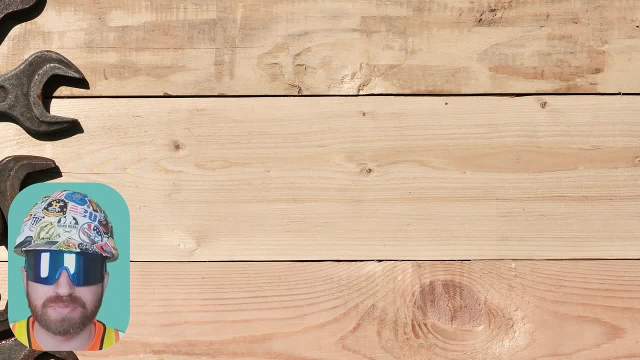 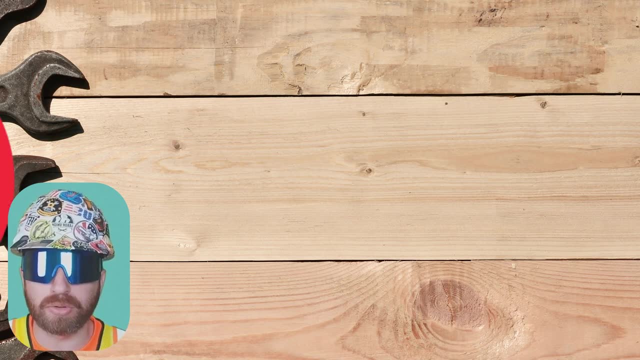 Now this might sound simple, but the importance of this statement is because many people create schedules where activities lack either a predecessor or a successor. These are considered open loops in a schedule that could lead to inaccurate overall durations based on logic driven in the schedule or your scheduling software. 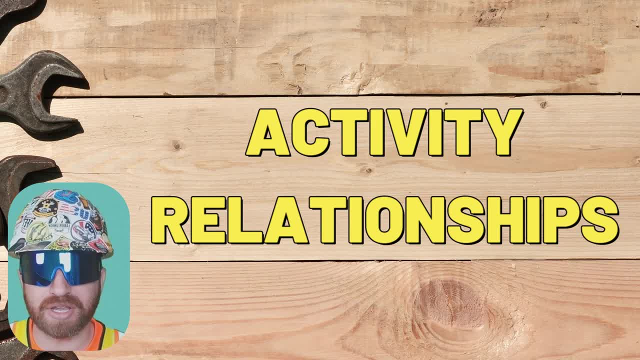 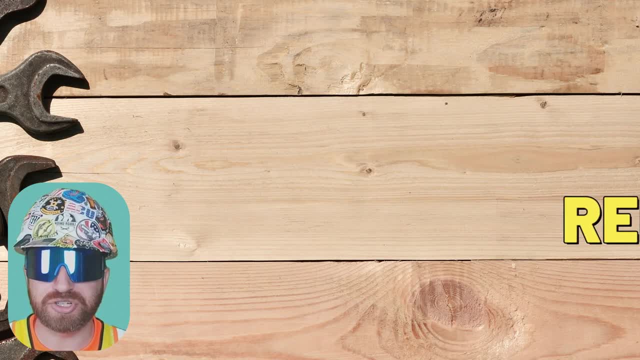 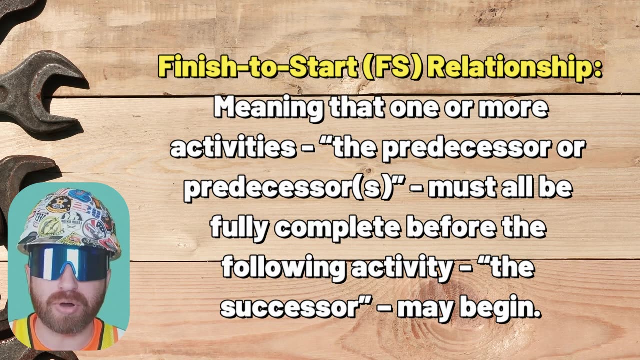 So I previously mentioned activity relationships, which is essentially how activities are tied to one another, and there are four of them. when it comes to scheduling, The first activity relationship type is a finish to start or FS relationship, meaning that one or more activities the predecessor. 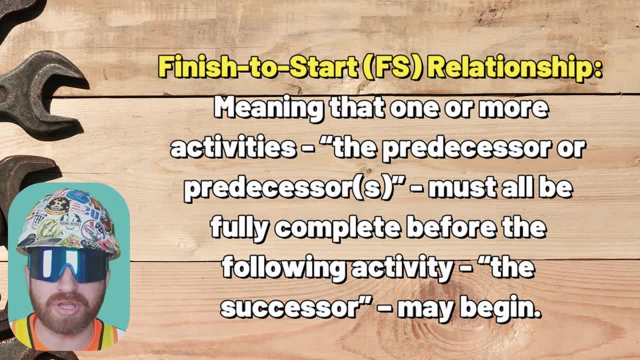 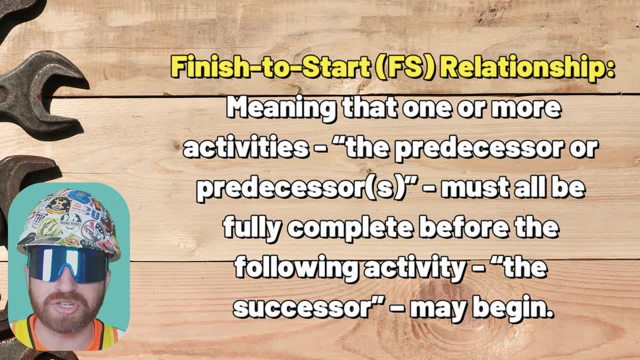 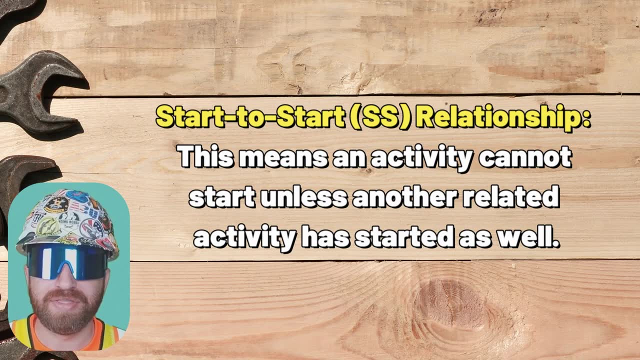 or predecessors must all be fully complete before the following activity the successor may begin. This is the most common type of activity relationship and we'll use this in our example shortly. Next we have a start to start or SS relationship. This means an activity. 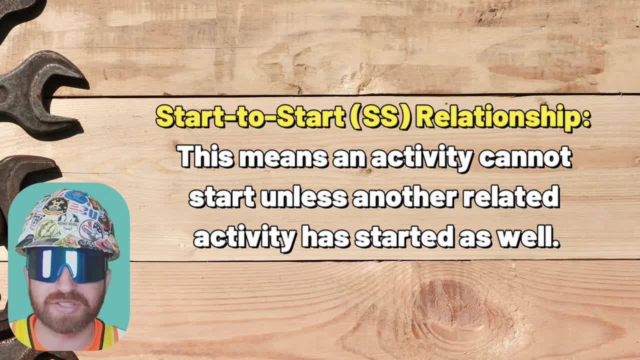 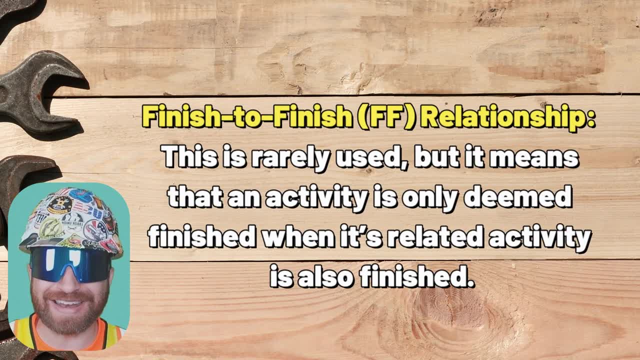 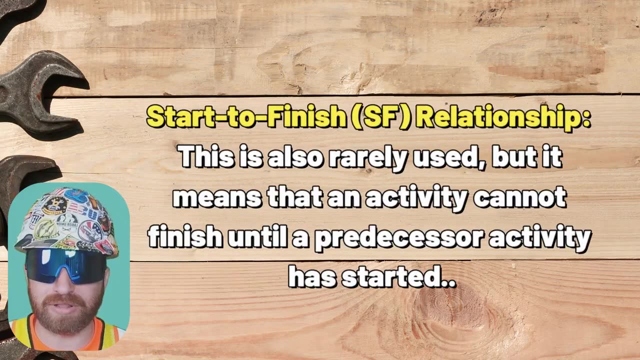 cannot start unless another related activity has started as well. Then we have a finish to finish or FF relationship. This is rarely used, but it means that an activity is only deemed finished when its related activity is also finished. Finally, the fourth and last. 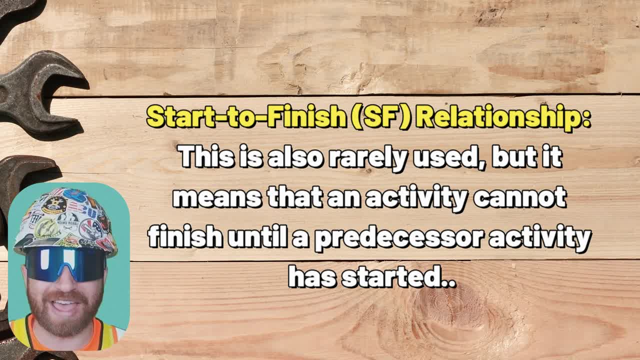 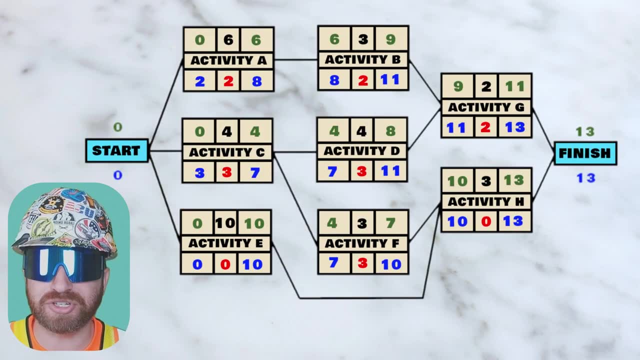 relationship type is a start to finish or SF relationship. This is also rarely used, but it means that an activity cannot finish until a predecessor activity has started. All right, so we've made it to our CPM schedule example Now. this example is a manual calculation. 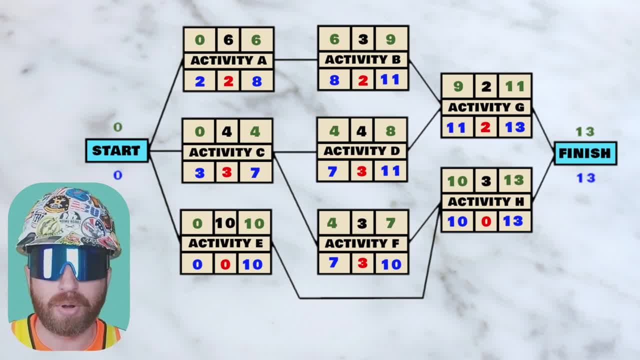 of what construction scheduling software will do for us. but we need to first understand how this will work on paper so that we can understand what's happening behind the scenes in our scheduling software, Once you understand how to manually calculate how a CPM schedule works. 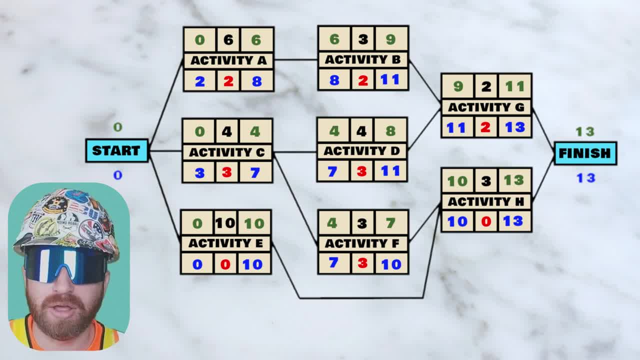 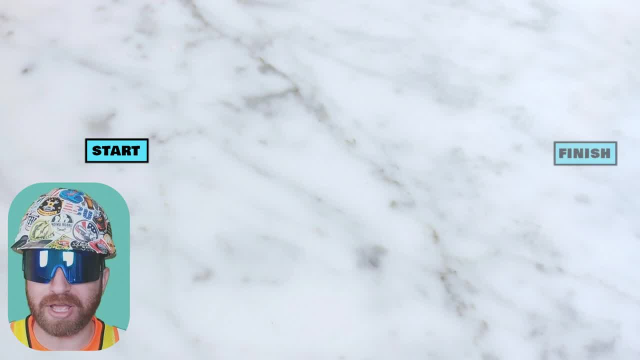 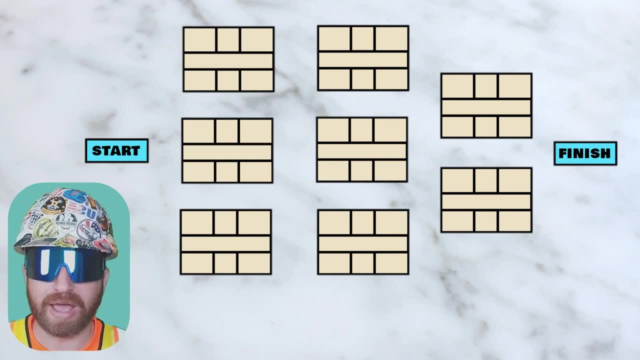 you'll likely never need to manually write out a schedule again, because your software is going to work 10 times faster. Okay, so this example has a starting milestone. This example has a finish milestone. This example will have eight activities in between, which I'll label activity A, B. 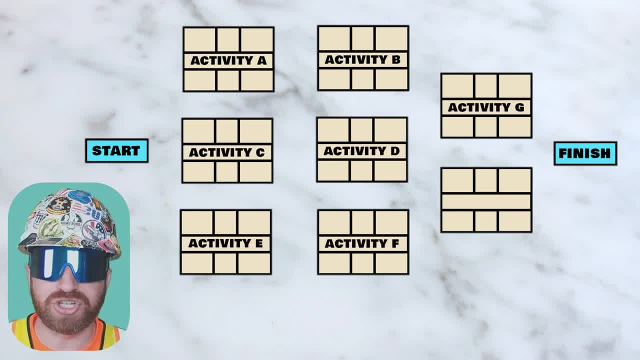 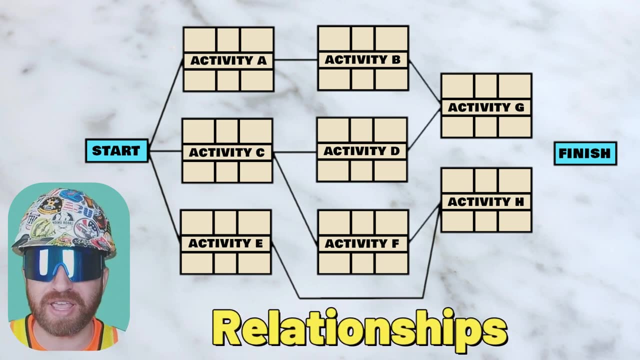 D, E, F, G and activity H. So I'm connecting these activities together with lines, which is how we would sequence this project as part of putting together this overall schedule. These lines represent the relationships these activities have with one another. Each line in this example. 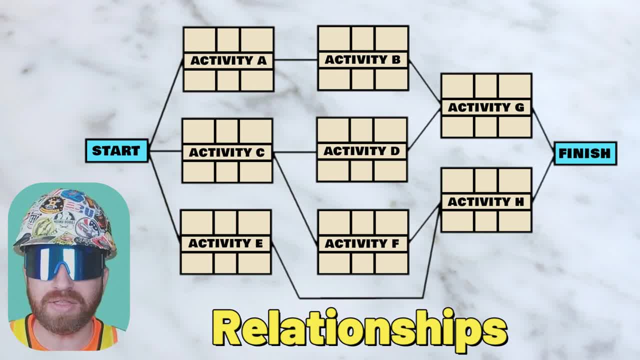 indicates a finish to start relationship, meaning that the successor cannot start until all predecessors have been completed. So, for example, if I have a CPM schedule, I'm going to have a start and finish milestone. This example, activity G, is a successor to both activities B and D. 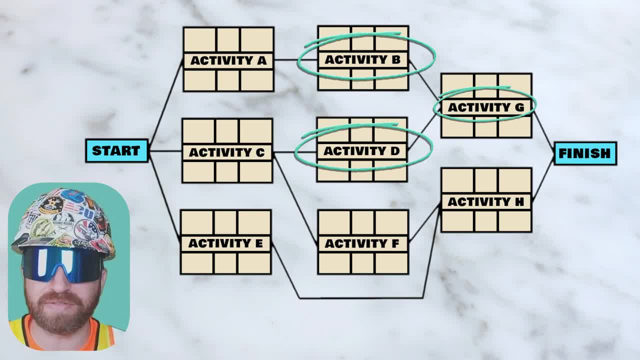 Activities B and D are predecessors to activity G, meaning both activities B and D need to be completed prior to activity G. starting Activity G is also simultaneously a predecessor to our finish milestone. Remember, all activities except our start and finish will have both predecessors. 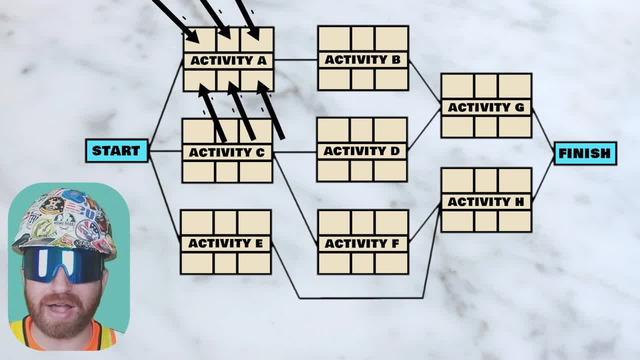 and successors. Now you see I have six empty зак blended out two-�로unda pieces of blank paper. So if I have a CPM schedule, I'm going to boxes within each activity which are going to be used to calculate our critical path through what. 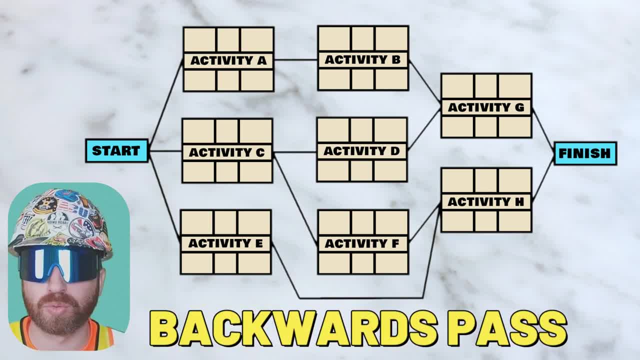 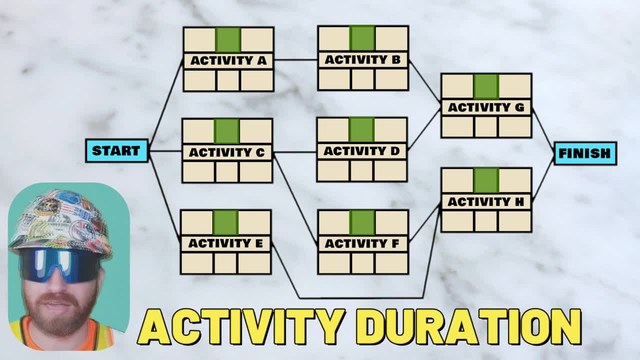 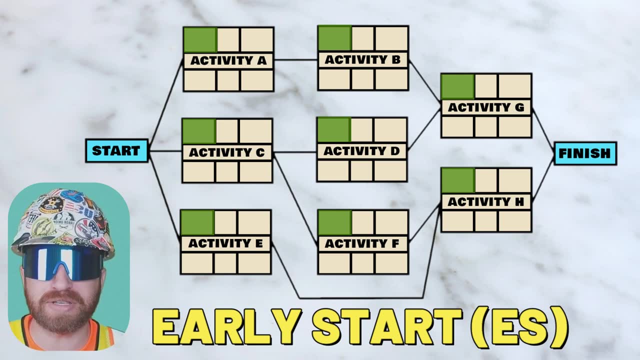 we call a forward pass and a backwards pass through the schedule. These boxes will represent each activity's total duration or time associated. These boxes will represent the activity's early start, or ES, as a number which is the earliest these activities can logically start, based on. 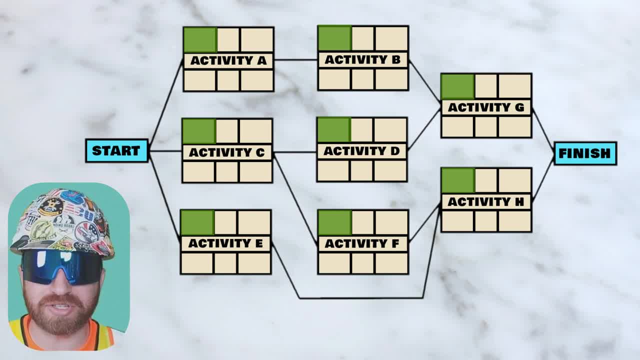 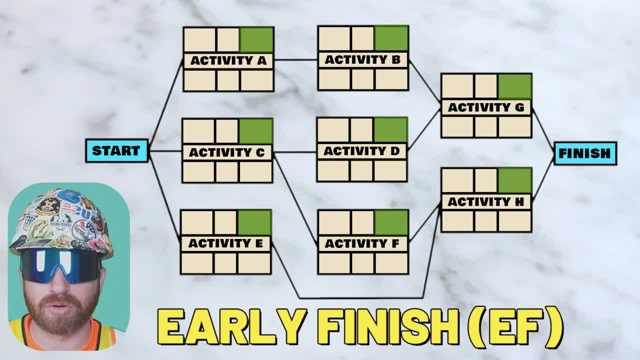 their predecessors finishing Again. this will all make sense in just a minute, once we start putting this all into action. so stick with me. we're almost there. These boxes will represent the activity's early finish, or EF as a number, which is the earliest these activities can logically finish. 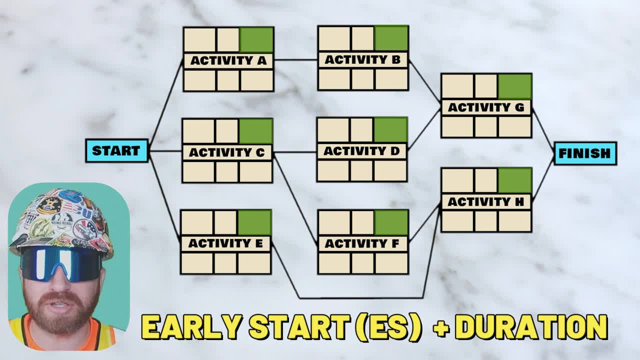 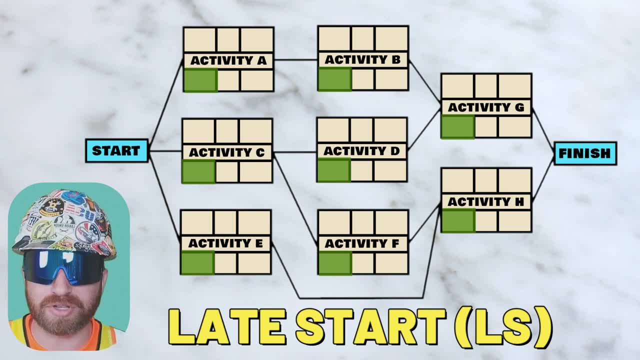 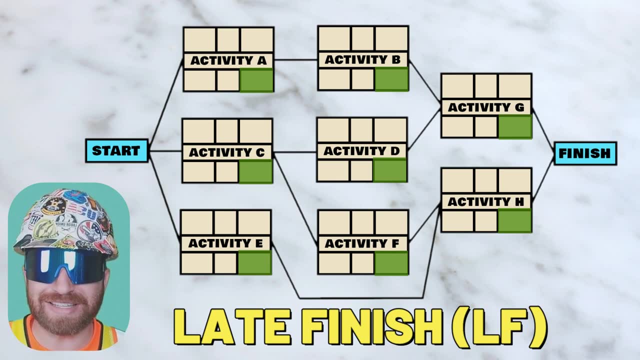 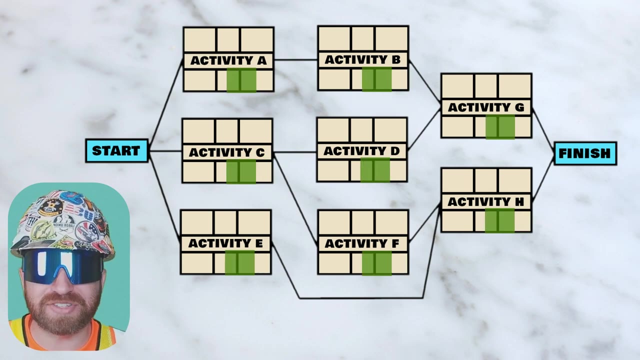 based on the early start ES plus the activity's duration. These boxes will represent the activity's late start, or LS, which I'll further explain shortly. These boxes will represent the activity's late finish, or LF, which is the latest these activities can finish without extending the end date of the overall construction project schedule. Finally, these boxes represent 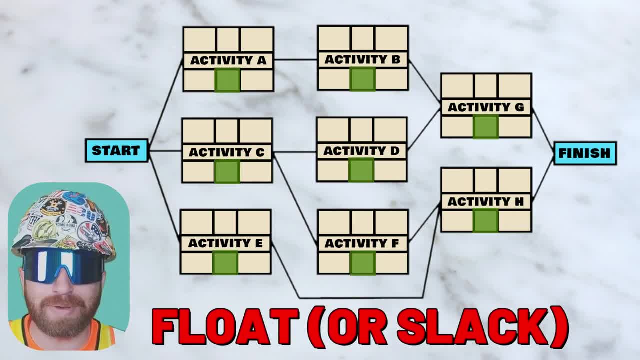 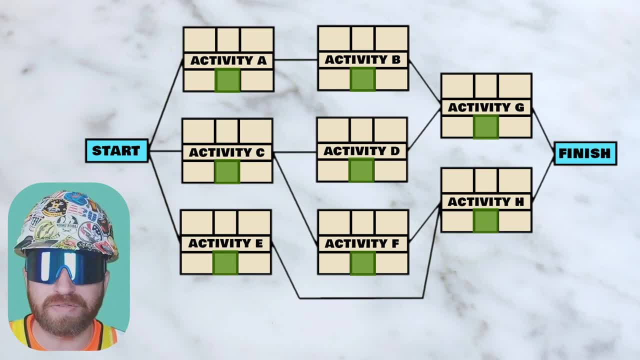 float, or otherwise known as slack, which is the amount of time an activity can be delayed without impacting the overall duration of the project. The critical path will appear when we've calculated the path that has zero float. So now we're going to start and we're going to manually find our 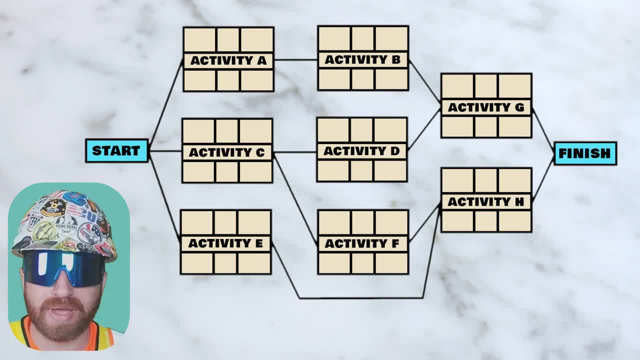 critical path by completing what we call a forward pass through the schedule. So let's go ahead and take a look at our starting milestone, and we're going to give this milestone a zero, because milestones do not have durations associated with them. So we're at our starting milestone and we 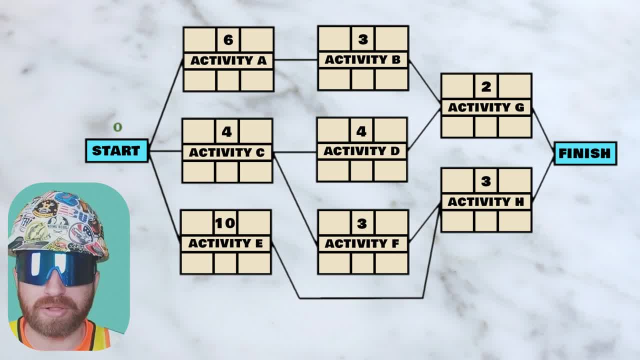 see that activity A, C and E are all directly related to our start, meaning that they can contribute to each individual activity. So we're going to start by adding in all of our start and end dates. So we're going to take a look at our starting milestone and we're going to 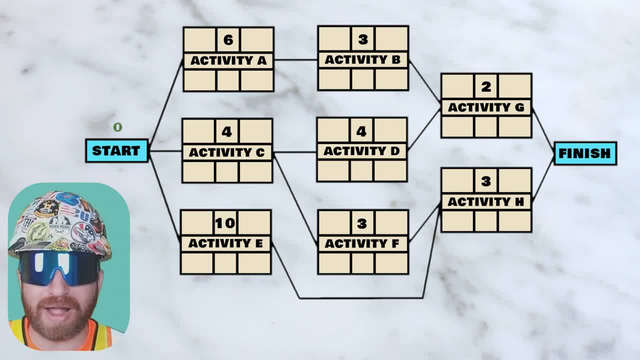 After our starting milestone has finished. Since our starting milestone has zero duration associated, these activities can start right away, meaning that their early start or ES will also be zero. So we've officially started our forward pass through this schedule. So if activity A has an 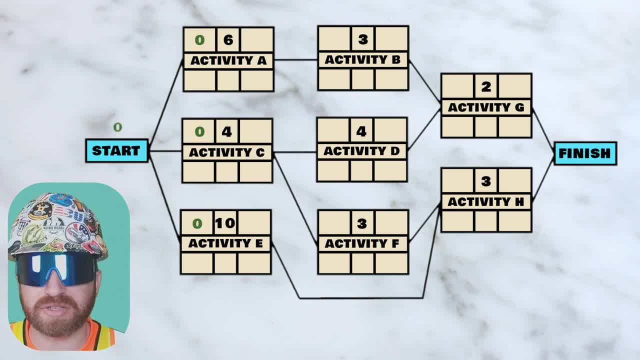 early start of zero and an activity duration of six. what is the earliest this activity can finish, otherwise known as the EF early finish? well, if we take our early start of zero and add our activity duration, which is six, we get a total of six. so the earliest this activity can finish is six days later. so we're 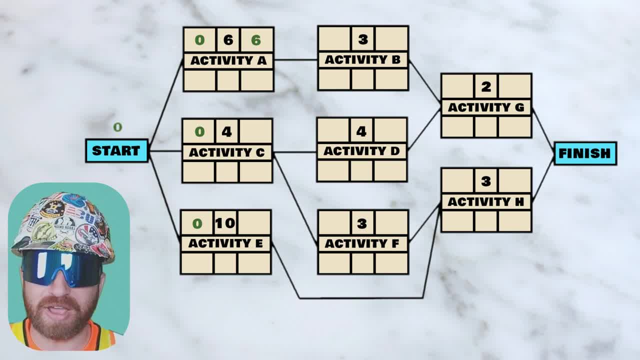 going to fill that in to our early finish date. next we have activity c, which also has that zero in the early start, but this activity has a four day duration, which means that the earliest it's going to be able to finish is at that day four, once we add our zero plus our four and we do the. 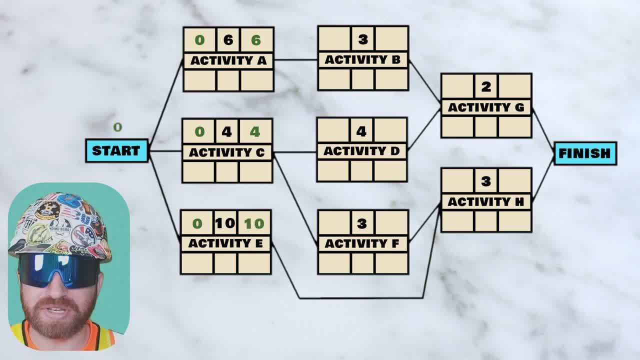 same thing, with activity e now jumping back up to the top. activity a has finished and its successor, which is activity b, is now able to start through the finish to start relationship. so activity a finished at day six, which means that activity b can technically also start on day six. so we carry. 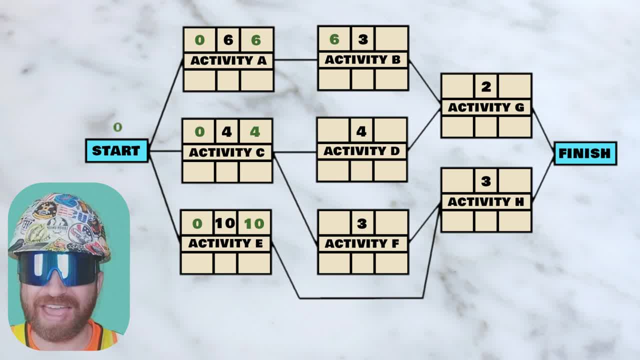 that through to activity b. b b's early start, activity d and f are both successors to activity c, so we carry the fourth through these as well. then we fall back and we do our calculation. for activity b's early finish, or ef, it started on day six. it has a three day duration, which means the earliest it can finish. 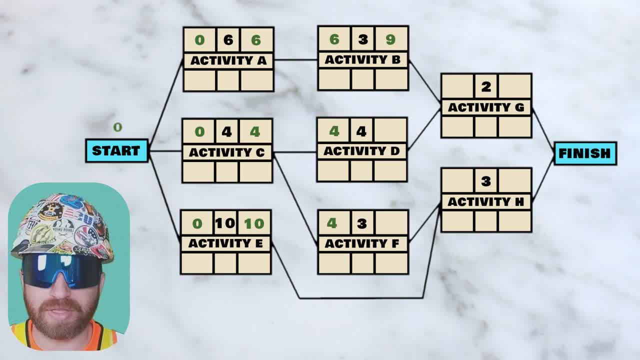 is on day nine. okay, so we do the same math and the same calculation for activity d and activity f. now what happens with activity d and activity f start? activity g is a successor to both activity b and activity d. this means that g cannot start until both b and d are complete, which means g is reliant on whichever activity of its predecessors. 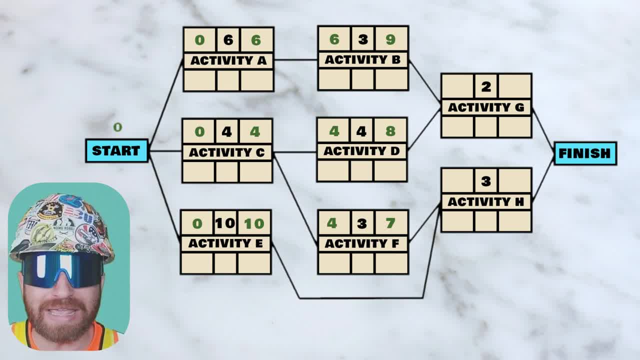 is going to take the longest, well, activity b ends on day nine and activity d ends on day eight, which means that activity g cannot start until day nine, since it's waiting on activity d, if activity b is gonna take the longest and activity d ends on day eight, which means that activity g cannot start. until day nine. since it's waiting on the activity b's early start, activity g, chapter four, is stop. if Eco got stuck at point e, sih going to lose Зевера ad gli ре Нитриfach. this means that activity gee cannot start until next time. activity ĹлъоðĤѢё γ vur. 왜냐하면 this activity Windows Finally start? 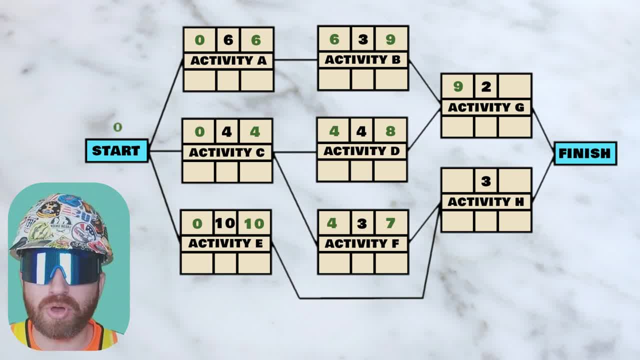 the longest activity to finish. now the same goes for activity h. its predecessors are activity e and activity f. since activity e has a longer duration, activity h is waiting on both to finish. but the earliest activity h can start is when activity e, the longer of the two, is wrapped up. 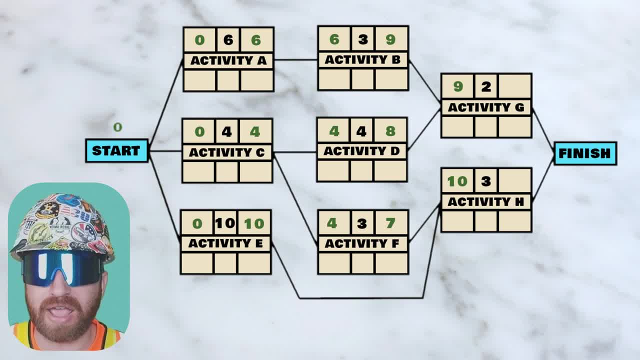 so we transfer that day 10 to our activity h, early start. now again we drop back and do our calculations. add day nine plus two days of activity, we get day 11.. adding day 10 plus three days of activity duration, and we get day 13.. so finally we're at our finished milestone. 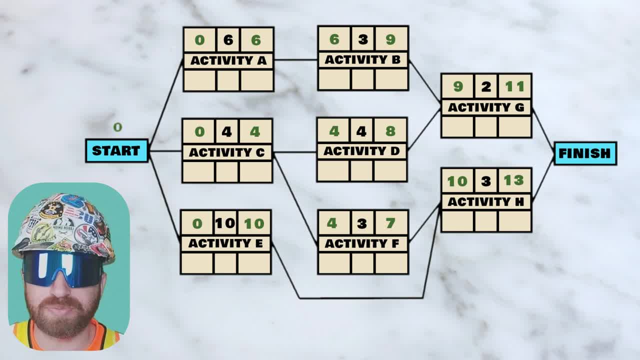 which is dependent on both activity g and activity h being completed. well, activity g can wrap up, but the project won't be complete until activity h is also completed. since h is ending later, then our finished milestone has to be associated with h, which is why we're. 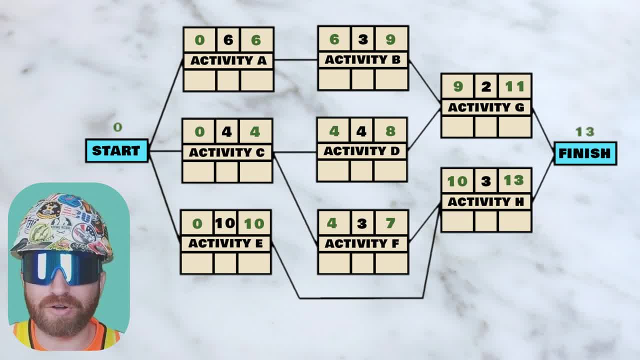 is on day 13.. so we've determined the length of our project by completing this forward pass, but we have not established what our critical path yet, so we have to complete a backwards pass. so essentially, we're just going to do the same process we did for the forward pass, but we're 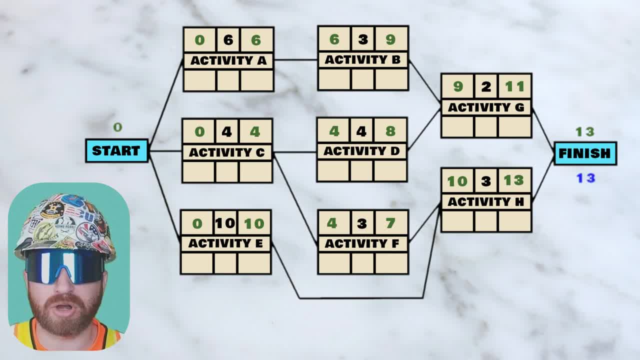 going to do it in reverse. so the top was our early start and our early finish. the bottom is going to be our late start and our late finish. so 13 is where we ended up, so we'll drop this in activity g and h's late finish. in order to calculate our late start boxes, we need to take our late finish. 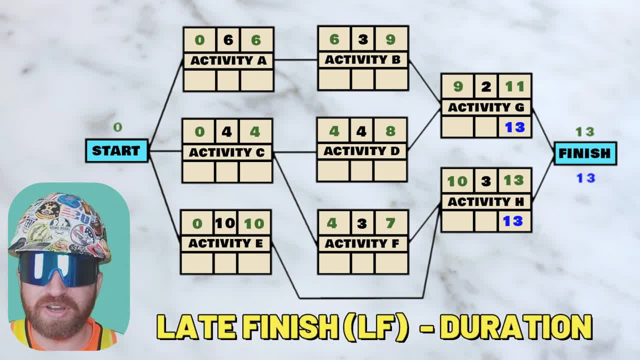 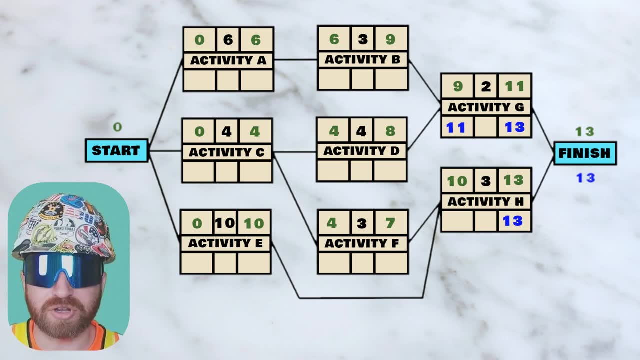 and subtract the activity duration. so for activity g, we'll take that 13 and we'll subtract our activity duration, which is two days, and we'll get a late start of day 11.. we'll do the same calculation for activity h: we'll take the late finish of day 13, subtract our activity duration. 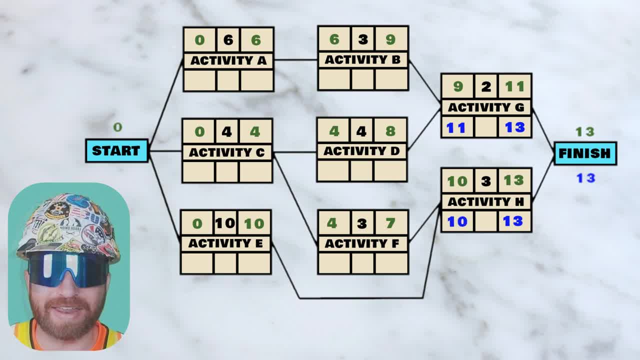 of three days, and we'll get a late start of day 11.. we'll do the same calculation for activity h. we'll take the late finish of day 13, subtract our activity duration of three days and we'll get a late start of day 10.. now we're just going to continue this process, working backwards with these same. 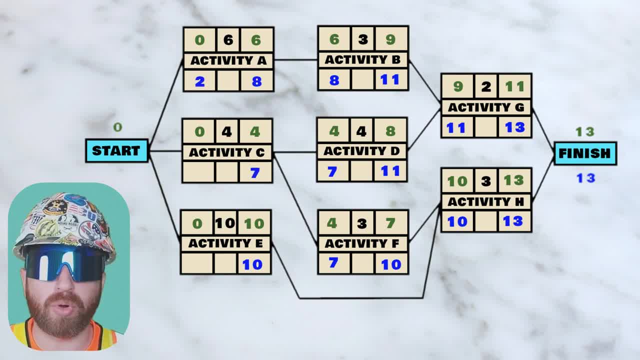 calculations through our schedule. okay, i've gotten to a point where i've hit three successors to one predecessor, but each of these successors have different late starts. so what do we do here? activity a has a late start of two, activity c has a late start of three and activity e has a. 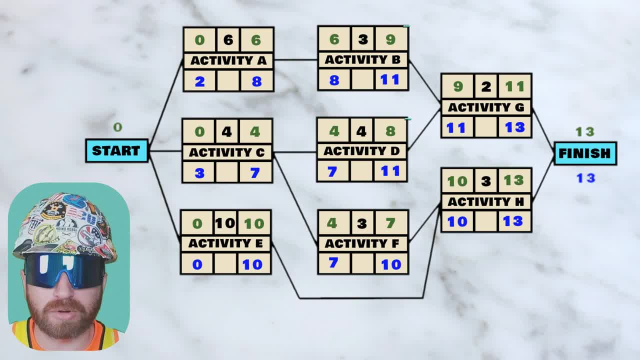 late start of zero. well, if you recall, on our forward pass we took the larger of the two when we were trying to figure out the early start of activity g. it's the opposite logic. on the backwards pass, we'll take the lowest number in any of these scenarios with multiple successors to one. 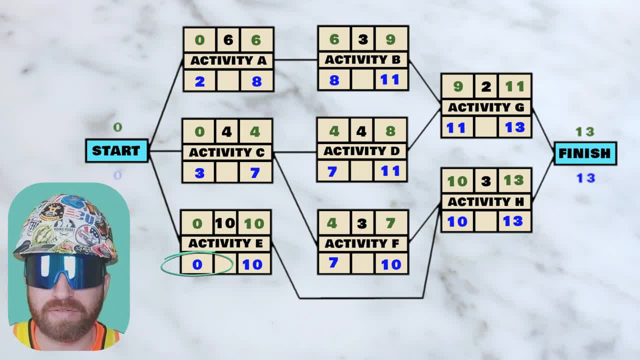 predecessor. so in this case we're going to take zero and feed it back to our start milestone. so we've completed both the forward pass and the backwards pass, which now has given us enough information to calculate this float and slack that i keep talking about. float or slack is calculated. by taking your late start and subtracting your early start. you can also take your late finish and subtract your early finish. so for activity a we're going to take two days less zero days, or eight days less six days and get two days. our float for activity a is two days. for activity b: 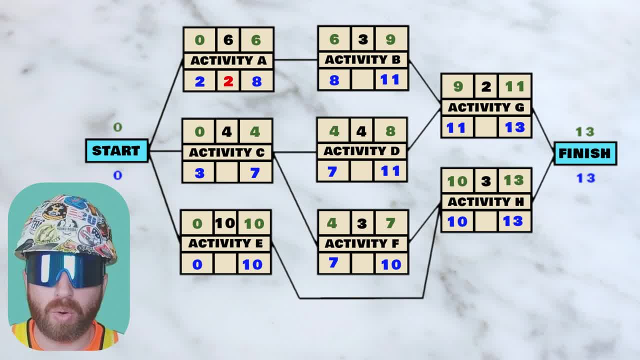 we take eight days less six days, or eleven days less nine days, which results in activity b having two days of float as well. so we calculate the float for all of our activities, which now outlines a path of activities with zero float or slack along its entire sequence. this is our 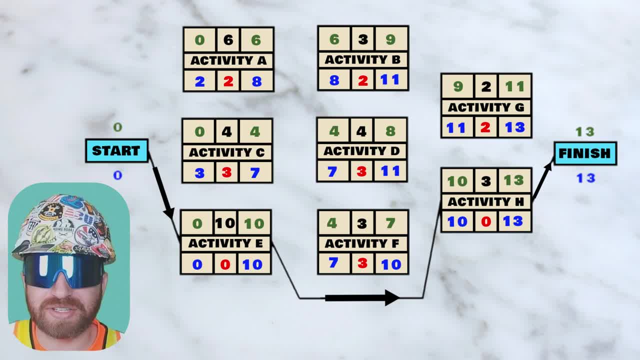 critical path on this project. so what this tells us is that if activity e takes longer than 10 days, takes longer than three days, it's going to directly impact and extend our schedule beyond these 13 days. so this tells me that we better keep a close eye on these activities if we want this. 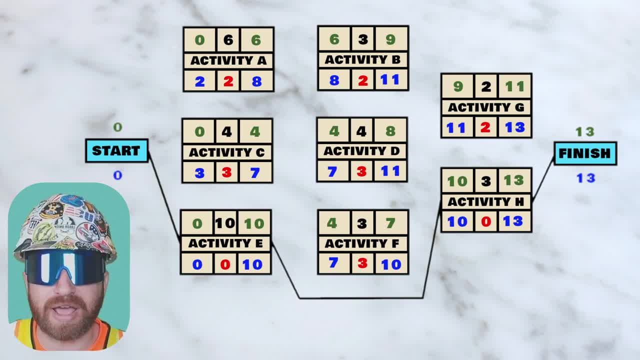 project done in 13 days, because these activities are not allowed any hiccups. so, on the flip side, every other activity in this schedule that is not on the critical path has float or slack associated with it after we've done these calculations, which means for activity a, activity a. 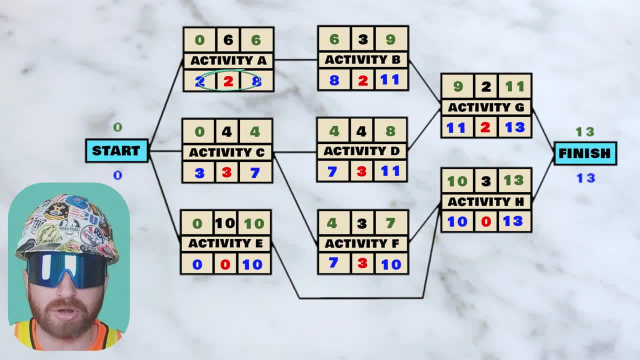 is going to be delayed two days after it was originally planned to start without impacting the overall end date of day 13.. it means that activity c can start three days after it was originally planned to start without impacting the overall end date of 13 days. this should now better explain. 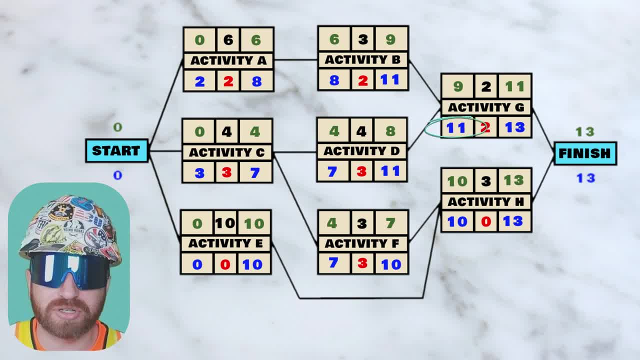 what a late start on the activity means. activity g doesn't need to start until day 11, for instance. however, if we use up more float than activity or sequence can afford, run the schedule update, our critical path is likely going to change and our project end date. 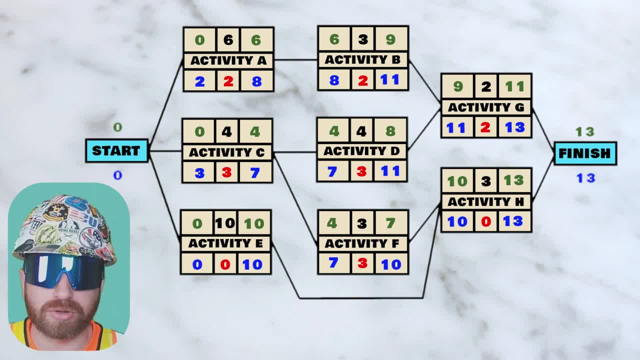 is likely going to change. The only way to recover on a critical path is to evaluate re-sequencing of relationships or to cut durations by using larger crew sizes. If you're working on a project and the schedule is not up to date, it's going to be difficult to determine if you're heading.